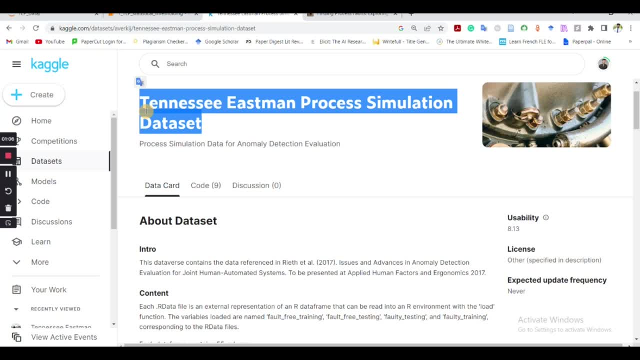 testing data. what are the faults? so basically, we'll try to get an idea of what this data set is and then we'll look further like how we can do again, how we can design a fault detection algorithm. for now we'll start with very basic, we'll start with the statistical method in this. 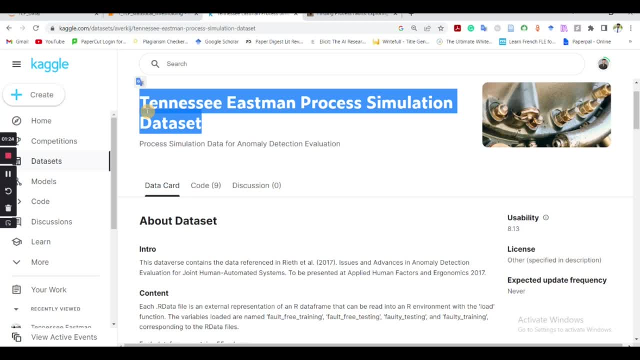 part one. as you have already seen the thumbnail, we'll use just basic statistical method and then we will graduate up to machine learning, deep learning and further and further we'll also. we'll also explore the xai, which is the explainable ai domain, as well, using this. 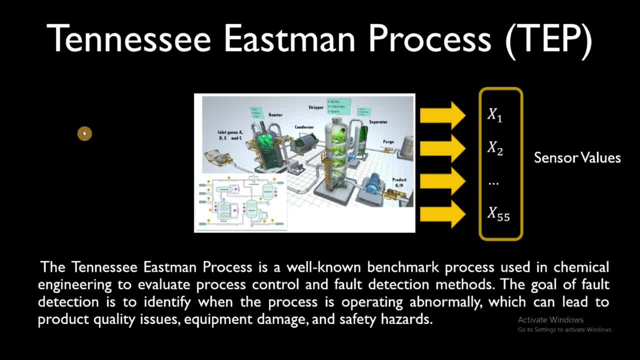 data set only. so, yeah, so this is the tennessee eastman process, and what we have in tennessee eastman process is a chemical plant. this is the entire chemical plant that we have. so so this is the chemical plant we have and from the plant we continuously 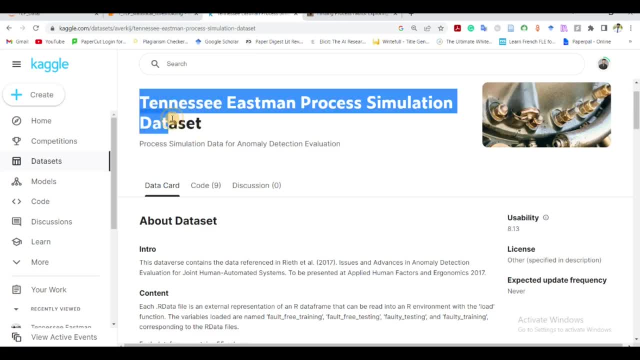 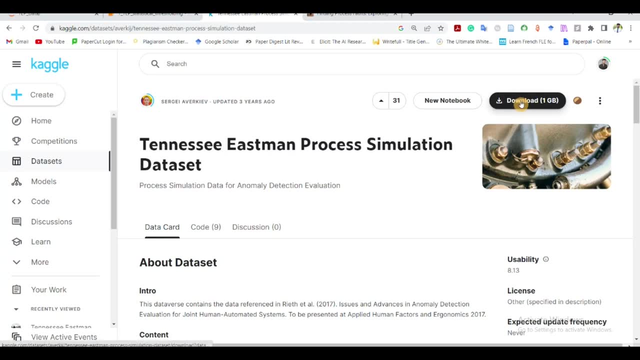 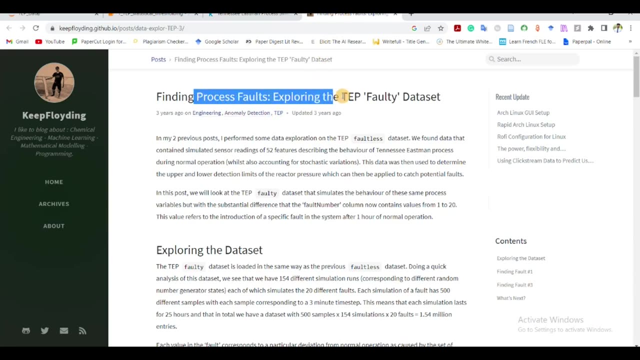 get some data and for the data set. i have got the data set from this gaggle website where the data set is open source and you can just download it and select one GB, but along with that i'll give you another source, this one finding process for exploring the complicator. so here they have explored the data set very well. 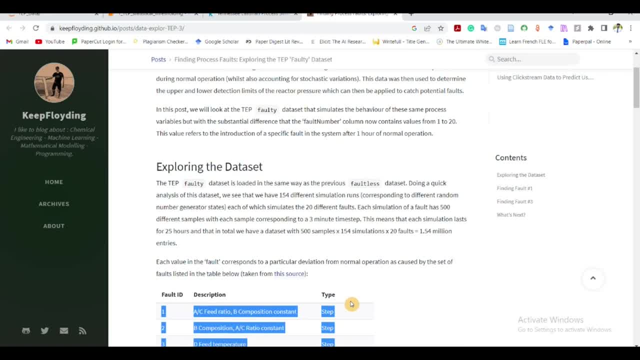 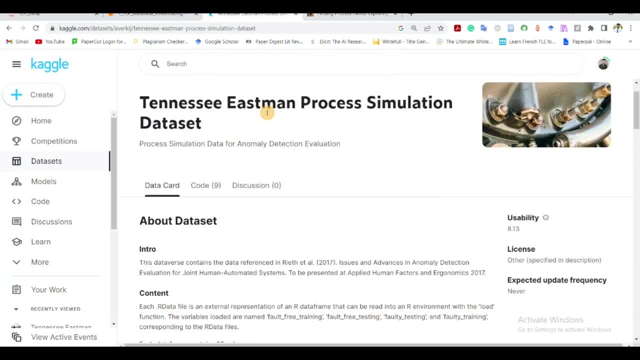 they have given what each fault means. how can you interpret that? and they have shown some basic detection methods as well. so your first task is to decent, that is, this is the investigation. are there in previous see? is our dvd? there are so many, then do I just go into theателей and give you the basic? 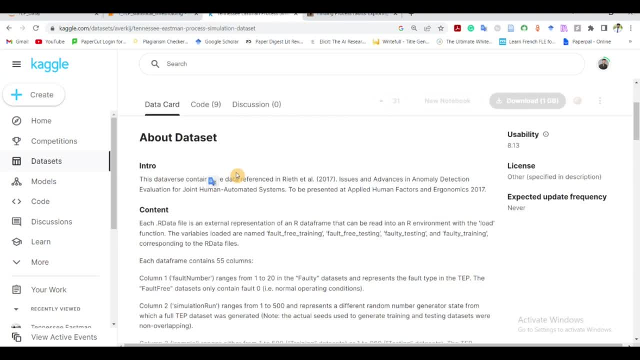 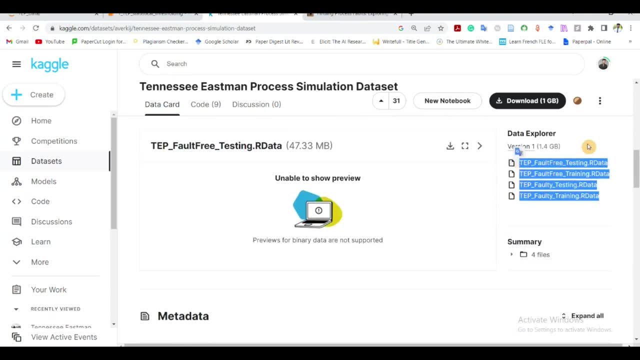 steps, which i will do using this large data set so you can hunt them. you can simply choose what白 dodge means. do you have these to go to here and download the data set? and the data set looks like this: it has. it is not a python file. you don't expect to see it in a python data frame, but this simulation was. 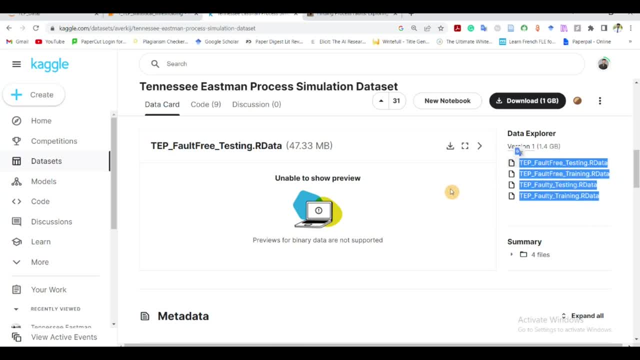 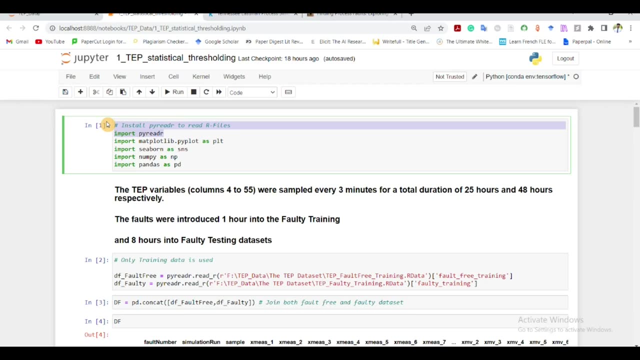 done in r. so this, all the files are in r data frame, and our first goal is to convert this r data file into python so that we can do our processing in python and so that what i created- this jupyter notebook and this is an important library you'll need to install- maybe you don't. 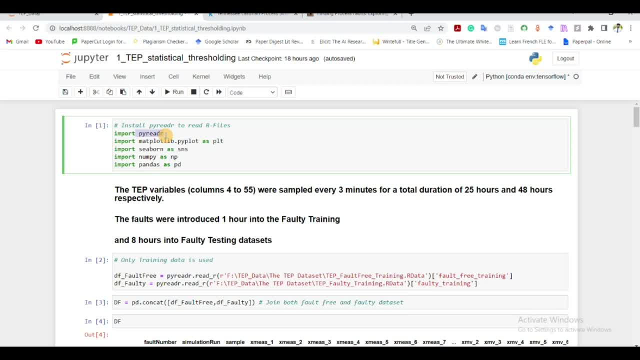 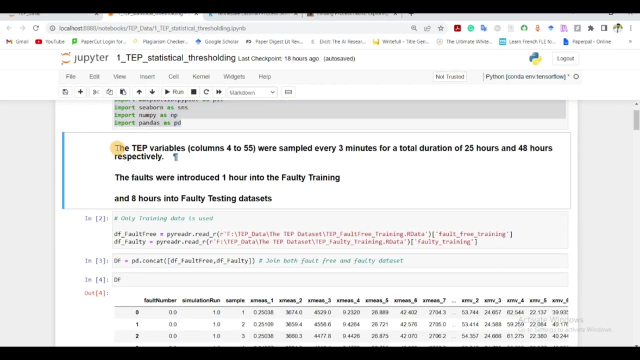 have that. it's called pyreader and this pyreader will help us to read the r data file in csv format. so, and this are rest of the usual libraries we always import, like matplotlib, c1, numpy and pandas. well, so give a brief introduction. we'll go to the. i've created a ppt. we'll go to the ppt to explore. 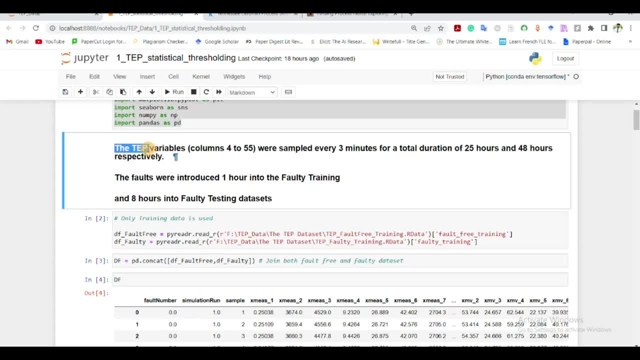 these details even more so. for now, the tep is the standard for tennessee eastman process, which is the process that we are exploring right now. so from for column 4 to 55 are the variables or the sensor readings, sensor measurements, and each sample was collected in between three minutes and for the training data set it was. 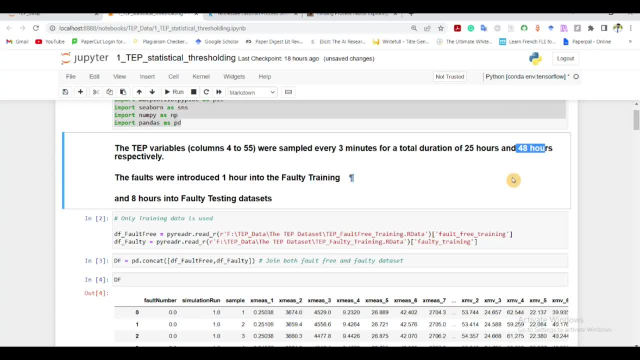 done for 25 hours and for the testing data set it was done for 48 hours. for the training data set, the folder introduced after our into the system, into the uh, once the simulation has been started, and for the testing dataset, it was started after eight hours. okay, for now, what we're gonna do is: 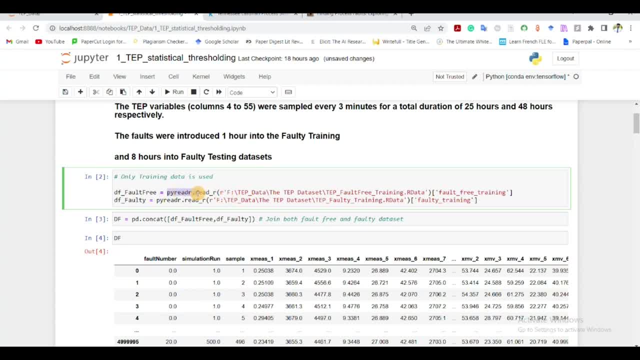 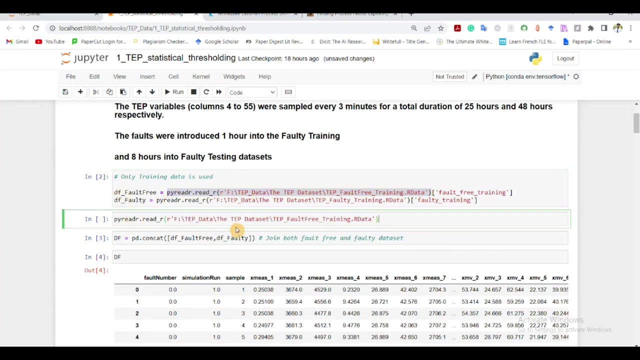 first you, uh, you release the function pi reader and, uh, we'll import, read r switch, will read the r data file and we'll give you the location from where you have the data file in your system. and then this is the key. this is the key within this, within this, is it? so I'll show you, I'll just copy this, and yeah, so. 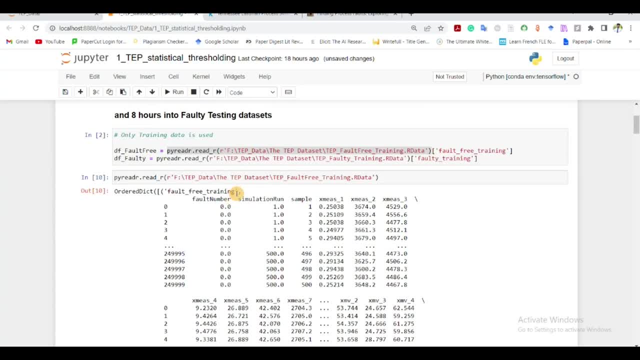 you see, this is, this is how the dresser looks like and this is the key that we need to extract. so that's what I'm putting this key here, and this is for the faulty training set as well, so that after you get the key, you directly get. 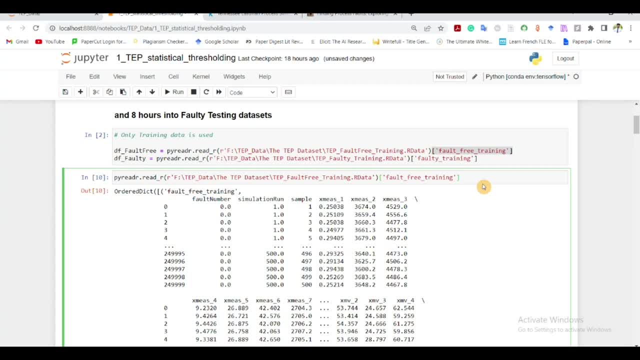 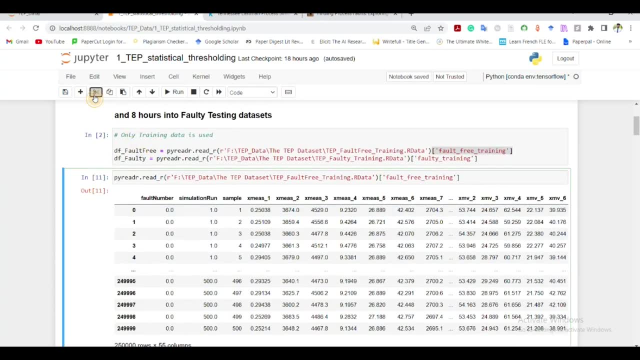 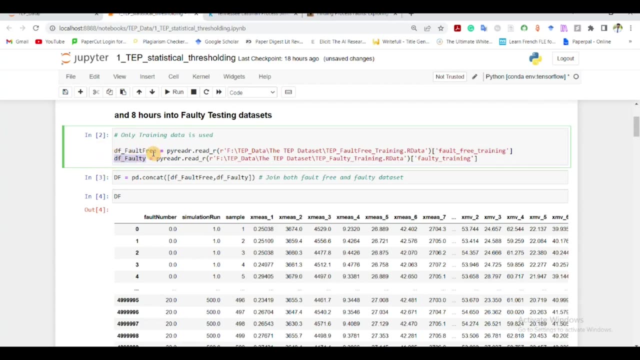 the data frame itself like this: so now you get the data frame which is our convenient, which is very convenient for us. so I did that for D a fault free and D a faulty, okay, and then what I did? I concatenated them both. fault pre has only data for fault free keys and faulty has data for all different kind of faults. 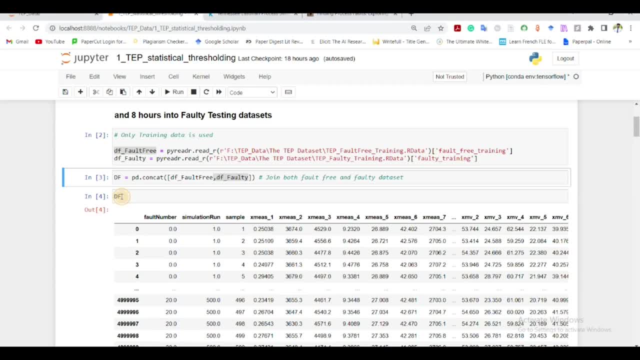 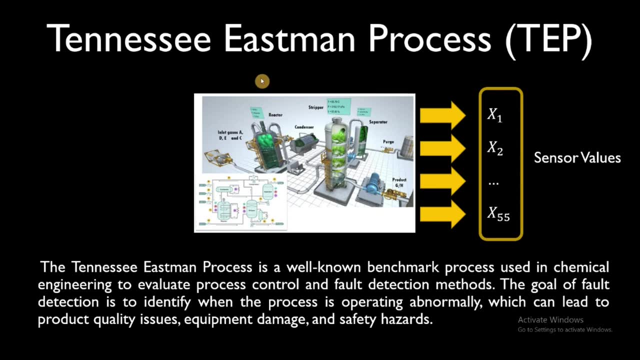 okay, so now that we got you a feel of what the data set is, let's see what this data set contents. okay, so in the Tennessee Eastman process we have the power plant here and we get some sensor reading. in this case we have 52 or 53 sensor values, doesn't matter. we 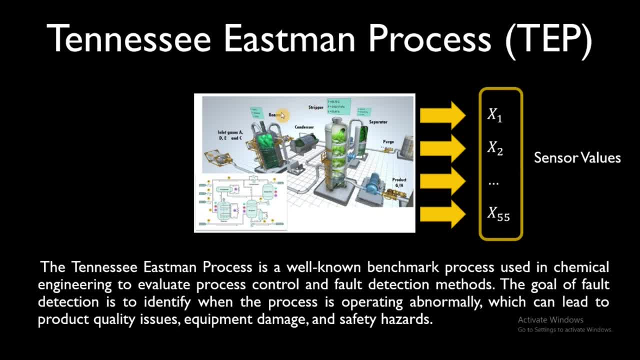 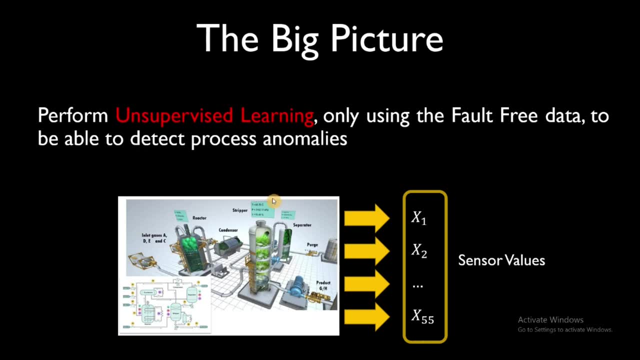 don't need to know what goes inside the processes. if you know, that's even better. but for now you're just going to share. analyze it in a perspective of a machine learning engineer, all right? so yeah, you 채. okay, so take you from the desktop that you were just working in and kind of 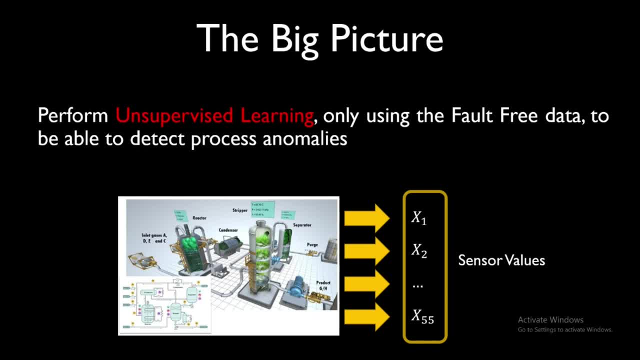 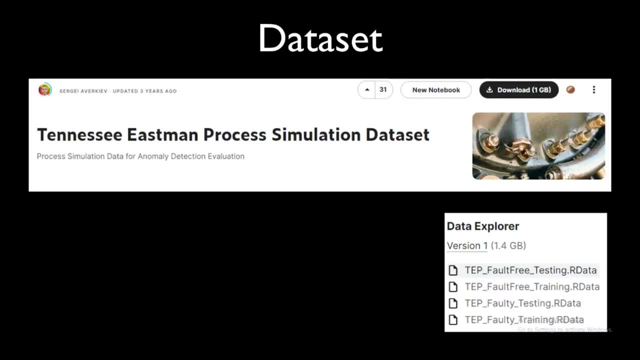 checking the items. so, yeah, and what is the big picture? well, doing what you want to do. so this is our system. we get sensor values from the, using the sensor values in an unsupervised method. we want to anomaly detection. so when there is a fault, we should be able to detect it using our algorithm and we don't need 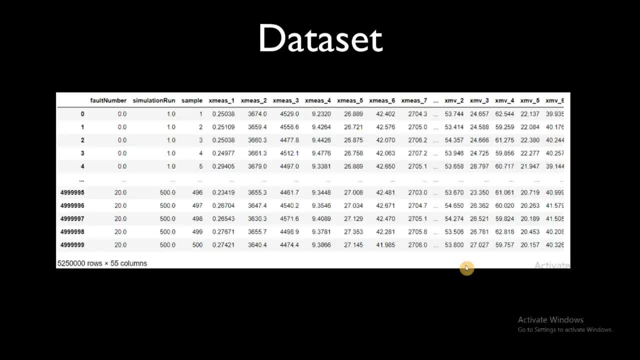 any labeled it up, because this is not supervised. love and the data, that is all r files. okay, this is. this is the screenshot of the data set that we just saw. the first one is fault number simulation run sample and, yeah, these are from xmea s1 to the last one. they are: 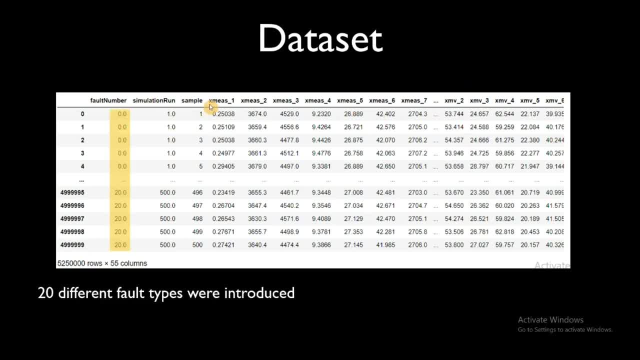 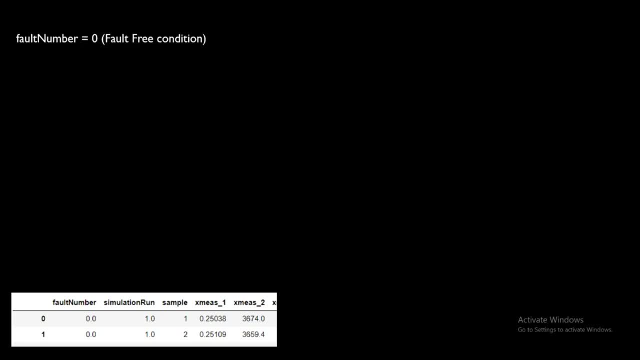 like 52 sensor values. so this is the fault, the different type of fault that has been introduced and 20 different type of follower introduced in there, indeed. so in the first case, we have fault number zero, which is uh, which is basically the fault-free condition, and in this, in this, 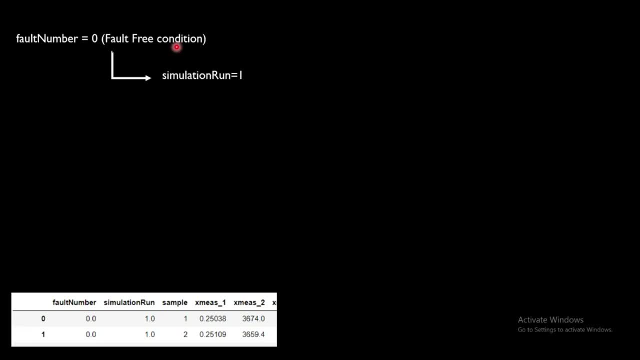 fault-free condition. we have different simulation run, so in every simulation you need to give some initial condition. in this case, the initial condition can be how much amount of material reactants are already in the tanks, something like that, and in different random initialization. they run this simulation for 500 different times and each time you have a different result. 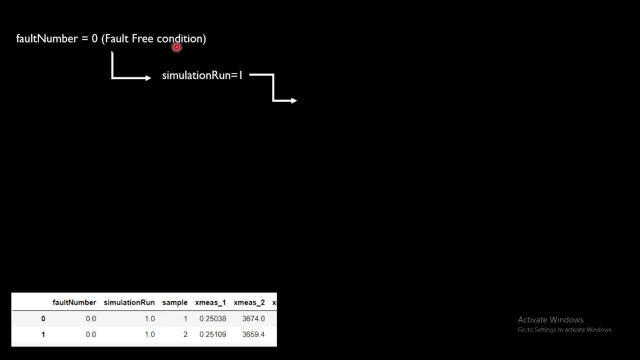 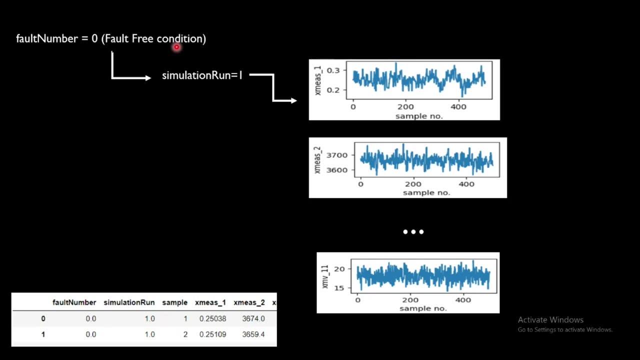 so in using simulation run one, and each simulation run has 55 variables, that has been monitored for 25 hours, and if you plot this according to sample number, you get something like this: and same has been done. uh, 55 different sensor values and same has been done for 500 times. 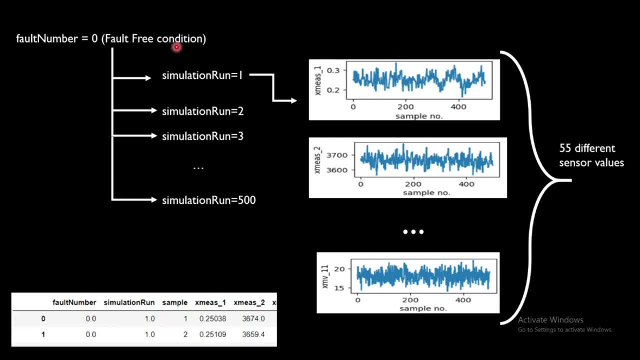 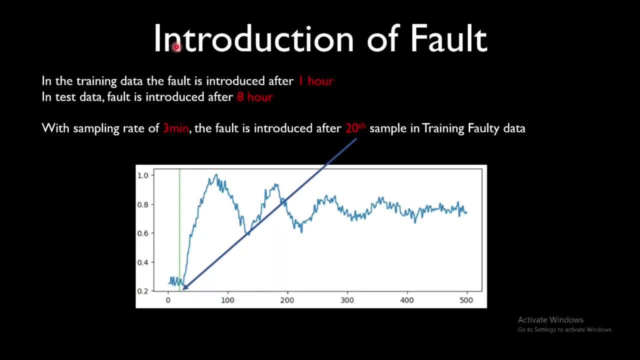 for each fault scenario. so that is an extensive amount of data we have from the simulation which you can use for our analysis. i hope that is clear by now. let's see introduction of fault. what time into fault was introduced? so in the training data which we are going to concern for now, uh, it has one hour, one hour into the simulation they have. 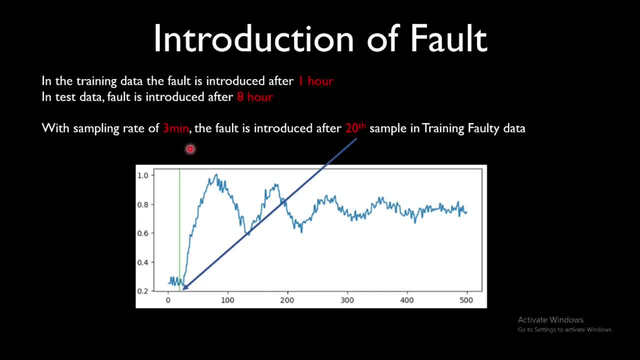 uh, introduced the fault. so what? what does that mean is the sampling rate was three minute. if you divide one hour by three minute, then we'll get 20th sample onwards. we get the order for this. so this is the year when the number went into the sample number that has. 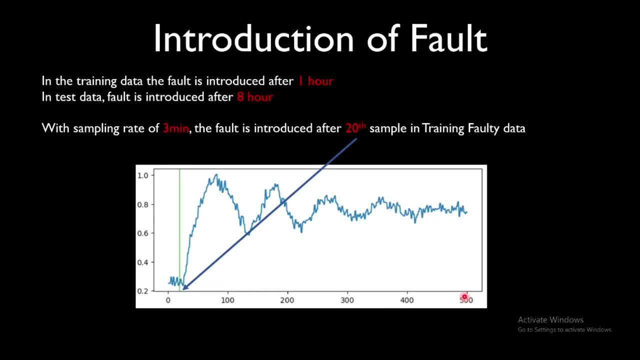 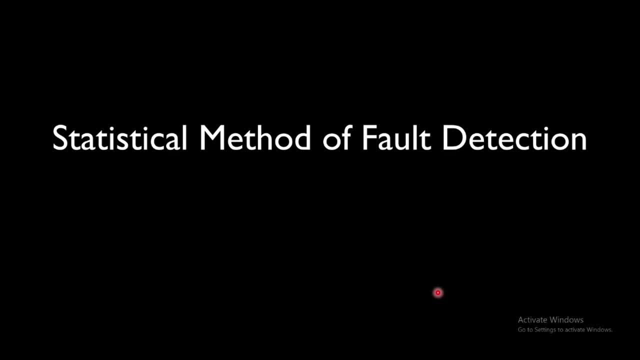 either became fault or jeunes has taken the fault. so this yellow, the green line, represents when the fall has started. basically, 20th sample. in the x axis you have the sample number, not the time, but the sample number. indeed, all right. so for for this uh, for this uh first video, we are going to use the 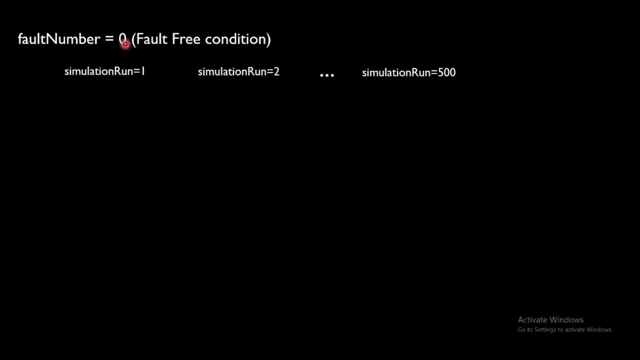 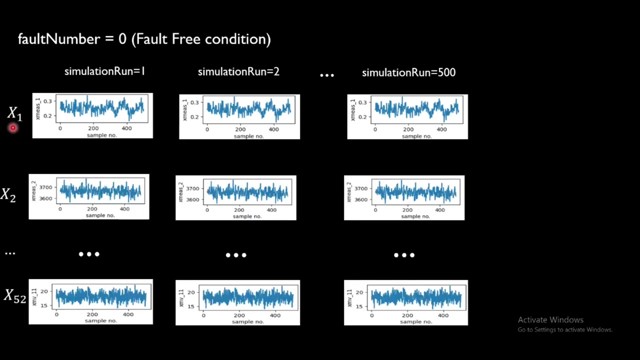 basic statistical method for fall detection and we are only going to use the fault free condition for that to simulation and 500. so we will get- uh, this is first variable we are- i'm calling them x1- and similarly you have like 52 variables. so what i'm going to do, i'm going to take 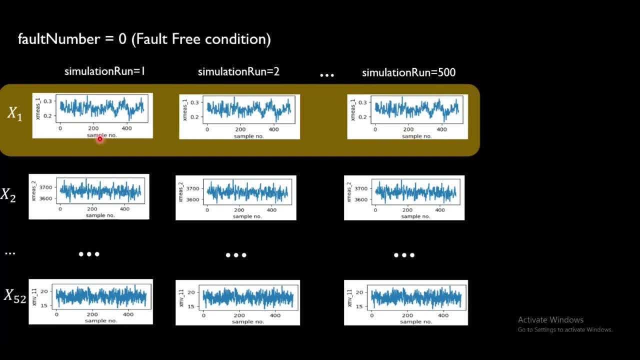 the first variable from 500 simulation run and plot it in a histogram like this. i am assuming that they belong to a normal distribution and i'm plotting them like this. and then i want the mean and standard deviation of this first variable. i'll call that mu 1 and sigma 1: same. 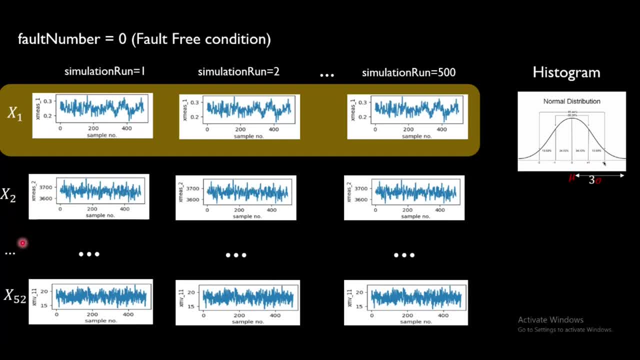 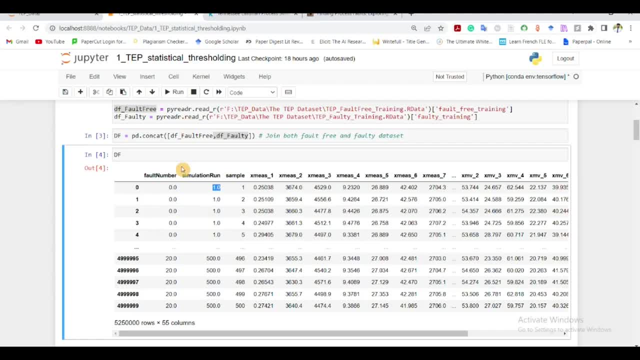 thing i'm going to do for each and every variable present in my fault-free data set. so i'll have 52 mean variables and 52 standard deviation variables. so let's see how we are going to do that. this is our data frame, which has all the data. 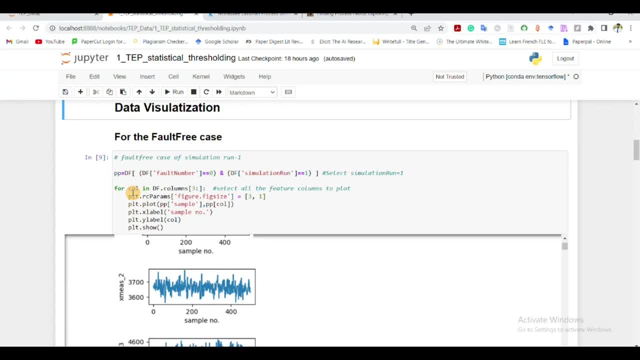 and next we are going to do data visualization. and for the fault-free case, especially if the data is of the, that is, of the normal scale. so what i'm going? pp is just like a temporary data frame, just for plotting sake. so what i'm going to do, i'm going to take my 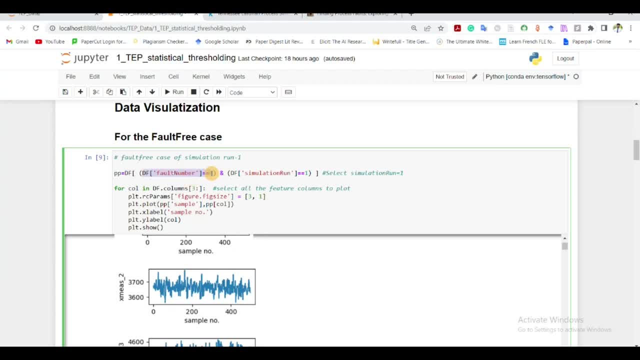 data frame, and in the data frame i'm going to filter that the fault number should be zero. that is the normal scale case, and i'm going to see for the first simulation run, how my data looks like exactly, and then i'm just going to plot it. 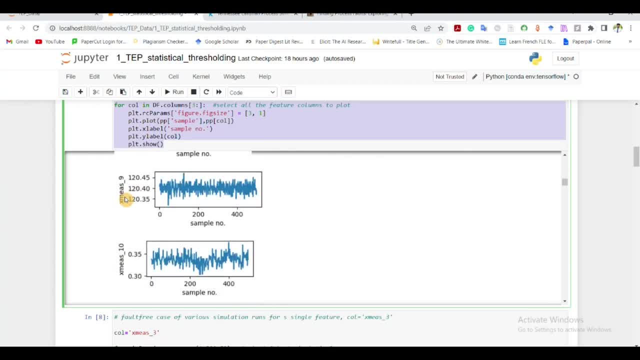 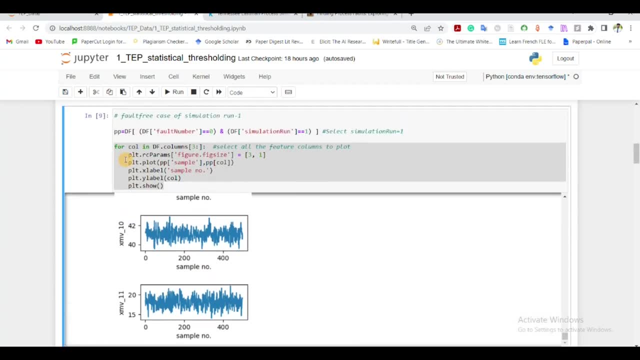 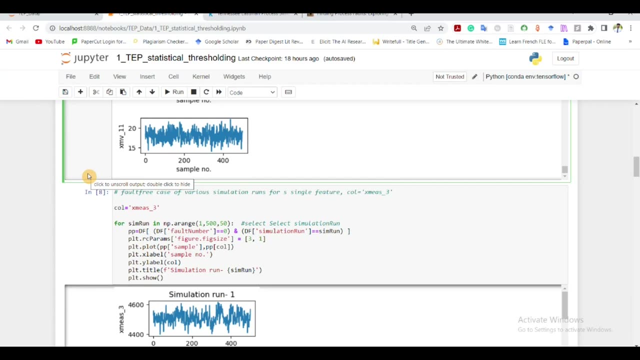 variable, for the second variable, third, fourth, fifth, sixth and so on and so on. so you get a lot of variables for just one simulation run, and this has been done for 500 times. this simulation run. all right, and then next, what i'm going to do, i'm going to see how the distribution looks like for 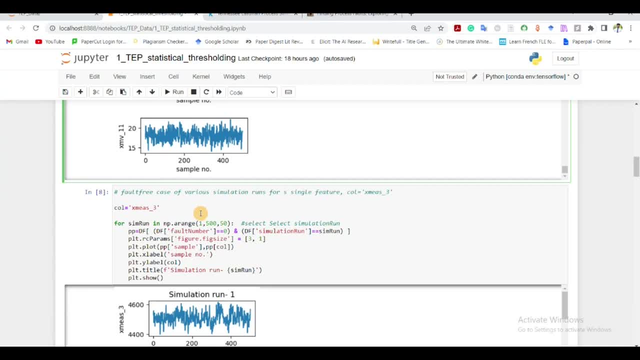 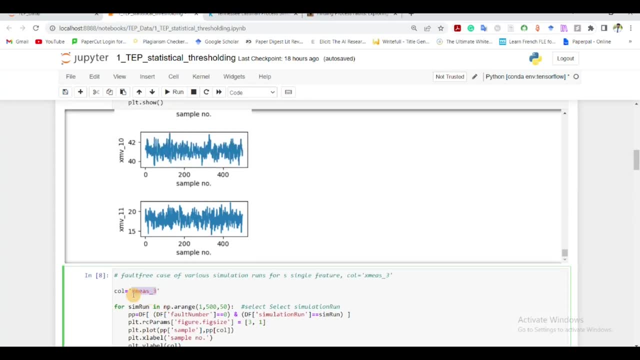 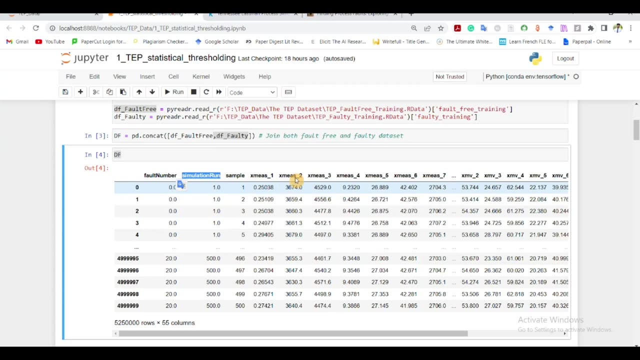 different simulation run for a single variable or single sensor data. so in this case, i'm choosing my column or the my sensor data to be xma3, this one, and i'm going to change different simulation run. like simulation run one. how does it look for this sensor variable? you can check. you can change this. 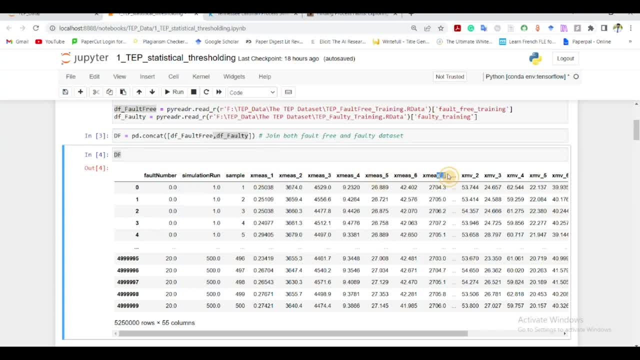 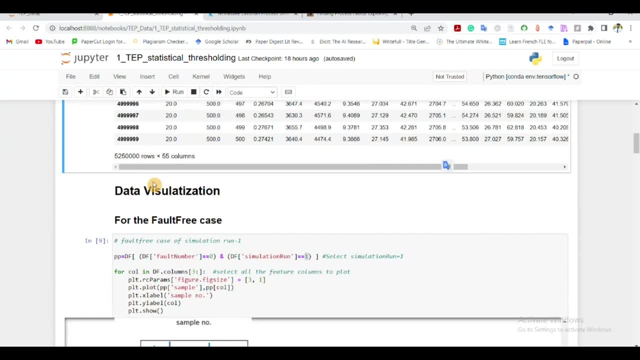 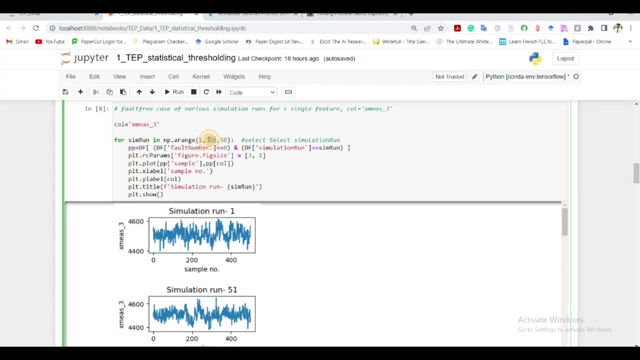 to any sensor variable. you can check this one, this one, this one, whichever one you prefer, and just see how it look, how it differs from different sample, from different simulation run. all right. so what i did is i i did a range from 1 to 500, with a gap of 50, so that i don't have to wait for a long time. 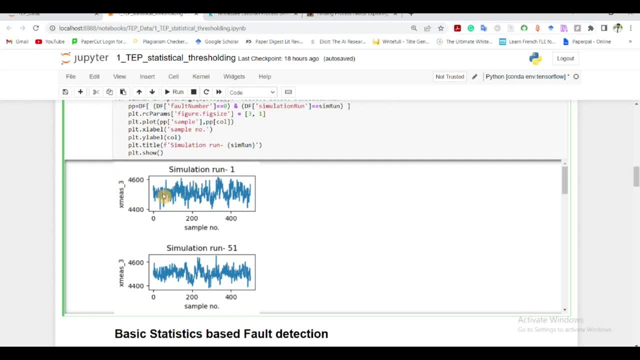 so this is for simulation run 1. this xma value looks like this for the range, you can see that it belongs to 440 to 460. in this case also the simulation run 51: it's same for 101: same. the range is basically the same. that's what i want to see and that for different values we can just 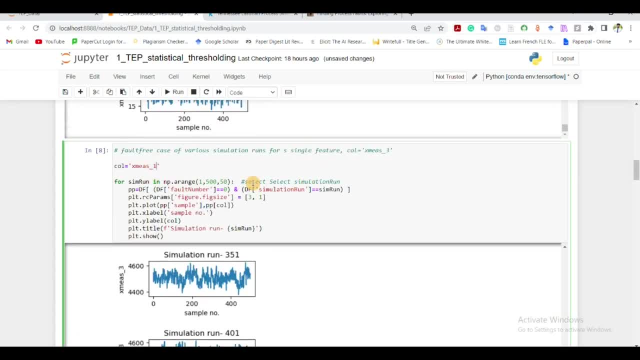 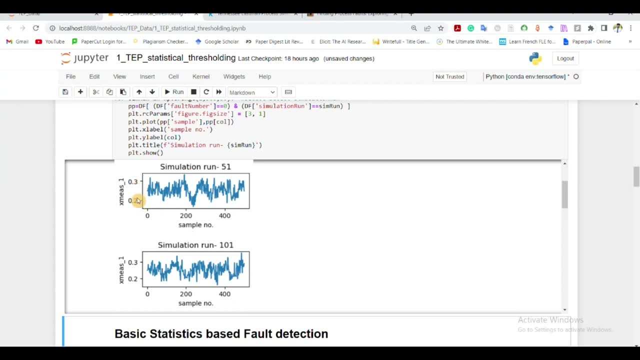 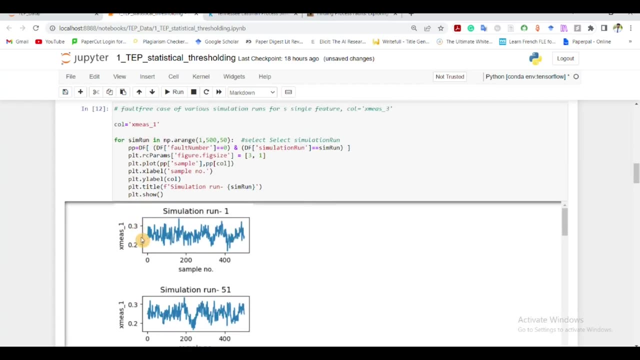 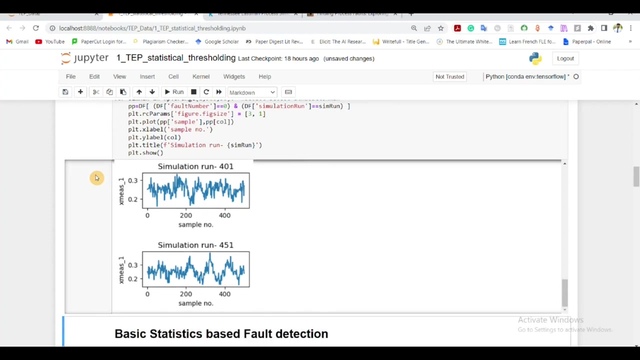 change that one to suppose i want the first variable, xma1. so yeah, here also. here you see, there is a big range in different uh between different type of uh sensors. so first sensor has a range from 0.2 to 0.3, whereas the previous one had 1000. that gives us an idea that when you try to do machine learning 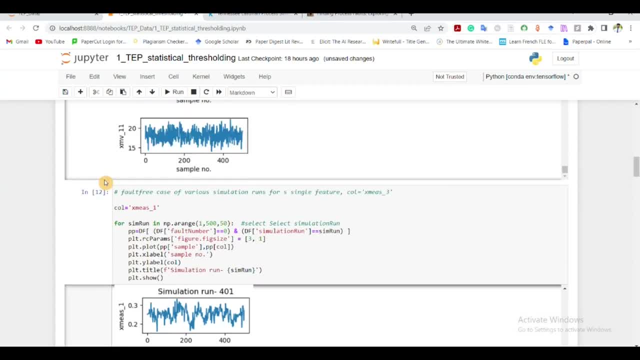 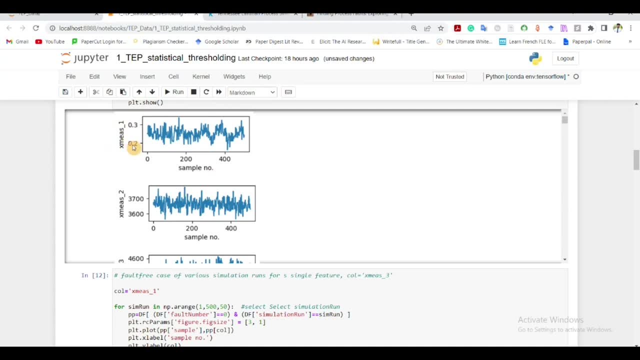 you need to scale these values, otherwise it will be difficult for machine learning to converge. yeah, yeah, here also you can see that. uh see, the first sensor has a range from 0.2 to 0.3. the second one has 3600 to like 3000. then 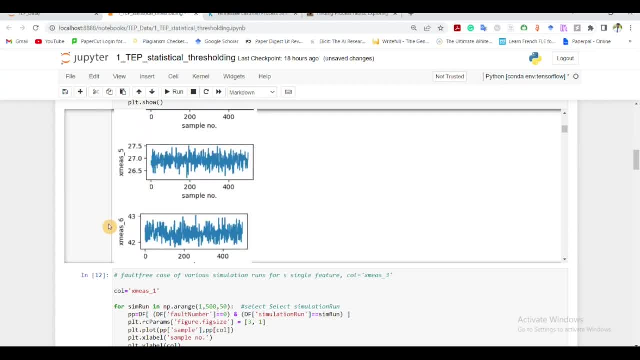 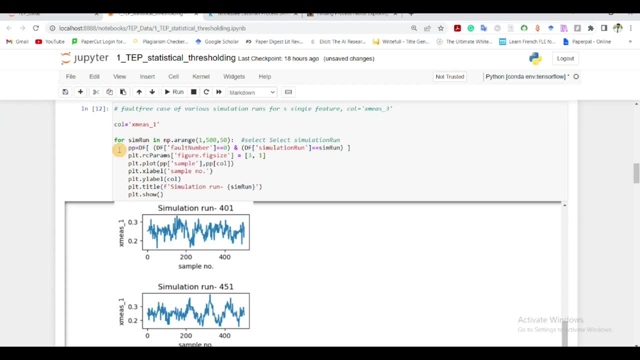 other is a 4000, then 9, 10. so, yeah, there is a big scale difference in individual sensor values, so we need to take care of that when you do machine learning. but for now it's good, it's well and good. well, now we did the visualization of how our data looks like. 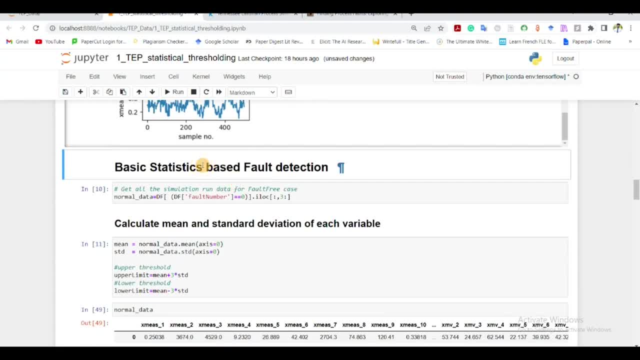 now what we're going to do. we're going to calculate the basic statistics, the mean and standard deviation. for that i'm going to create a temporary data frame- normal data- where i'm i'm going to take the 500 simulation run data only for the normal condition. i'm going to take all the data from. 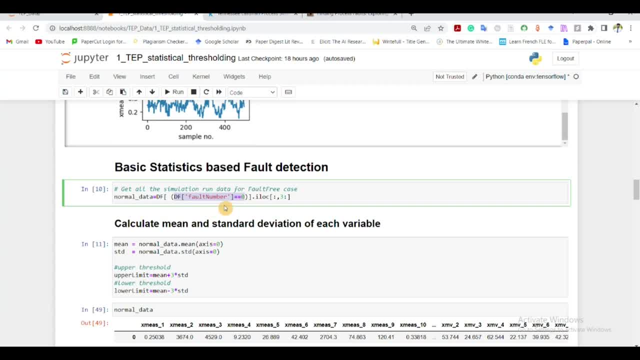 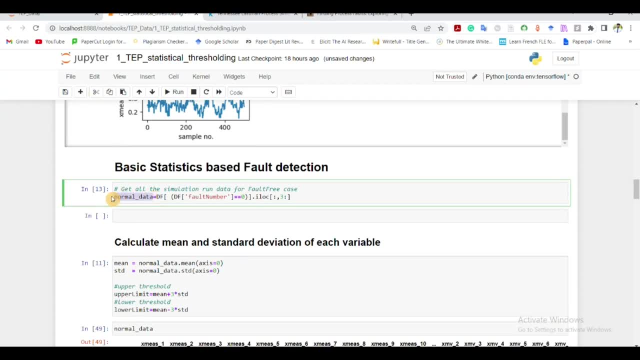 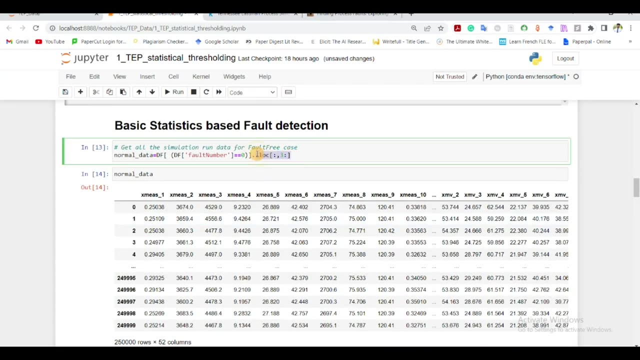 the normal condition, uh, fault number 0, which is the normal condition, into the normal data frame. and if i see how the normal data frame looks like, yeah, so in the normal data frame. uh, i also deleted the first three, uh, first three column because you know i don't need them for the 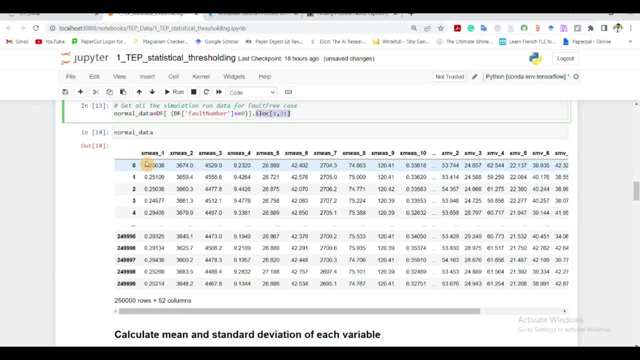 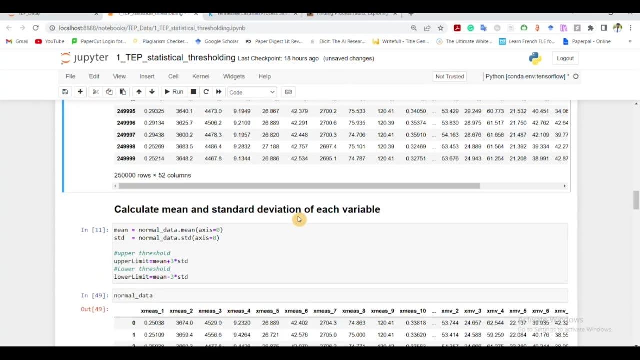 analysis and this is the normal data. so, uh, all right. so what i'm going to do, i'm going to take the uh mean and standard deviation of each column, each column, and then i'm going to analyze this, so calculate the of each variable or each column. so, using this mean and standard deviation, 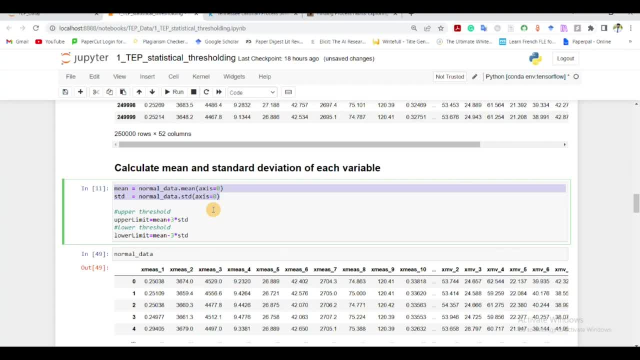 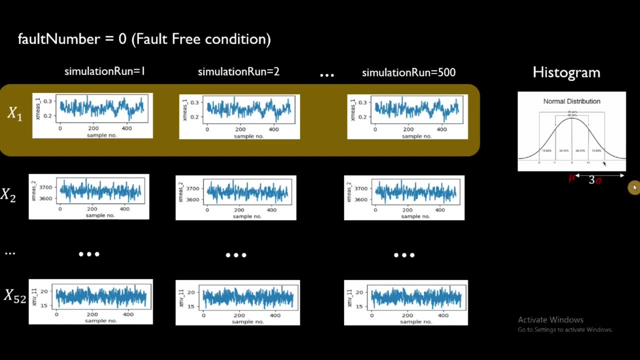 of the data frame, of the pandas data frame, we can just get the mean and standard deviation and then what is upper limit? is so mu plus three sigma will be your upper limit, which will correspond to 99 of your uh normally distributed data, and mu minus three sigma. 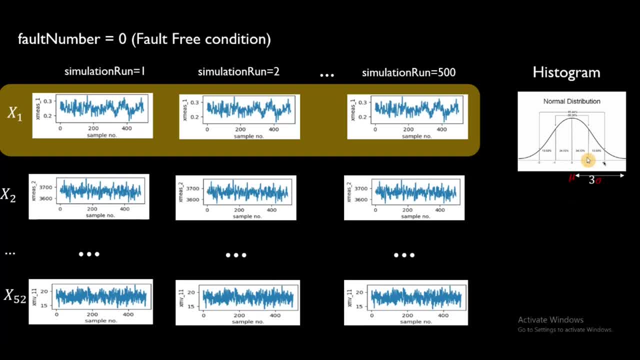 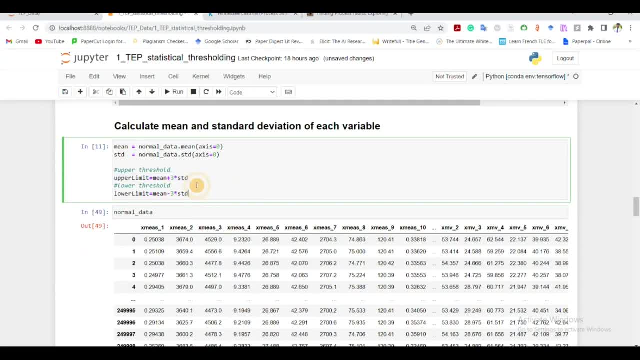 will be the lower limit. so our data should in the normal, in the normal scenario, it should range between this six sigma range. okay, i think that is clear now. uh, so upper limit is mean plus three standard deviation corresponding to 99 of the data, and mean minus three three. 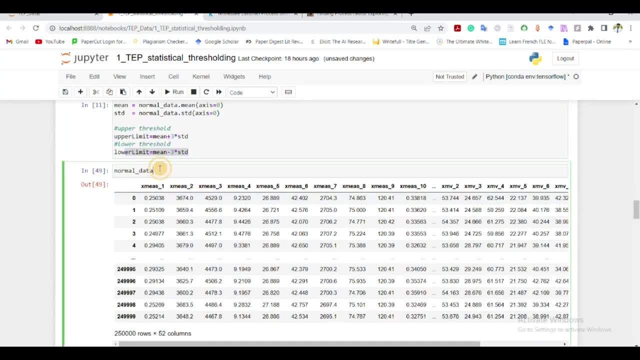 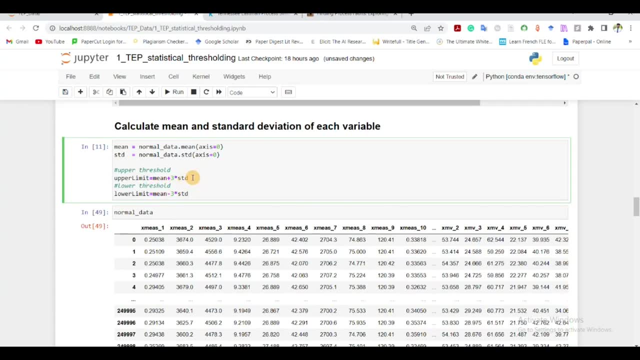 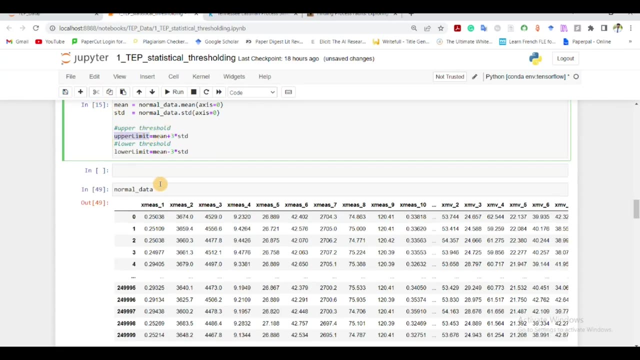 standard deviation. all right, so normal data is this, and then what we're going to do is now. now it's the interesting part, this thing: we already got upper limit and lower limit, so let's see what is my upper limit is my upper limit should be a. it is a 52 length variable. 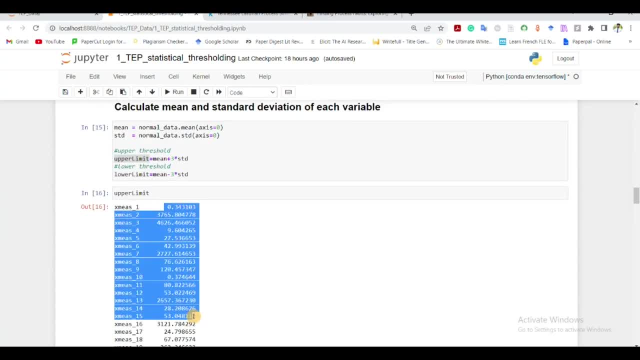 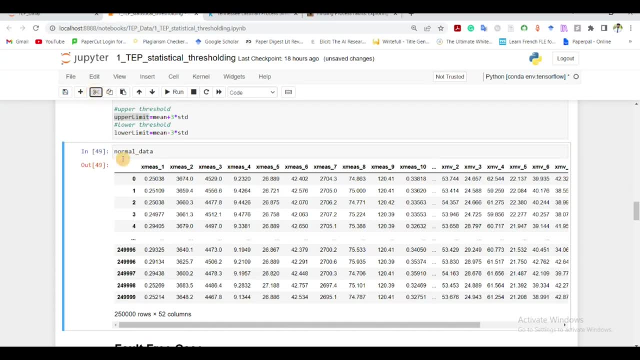 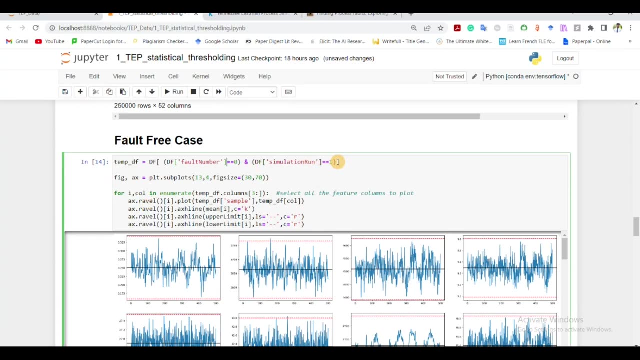 where it captures the upper limit of each, each variable, each variable as in each sensor data, and same is for lower limit. and now what i'm going to do? i'm going to use this upper limit and lower limit to do a monitoring. well, so what i'm going to do, i i'm just again importing the normal, normal. 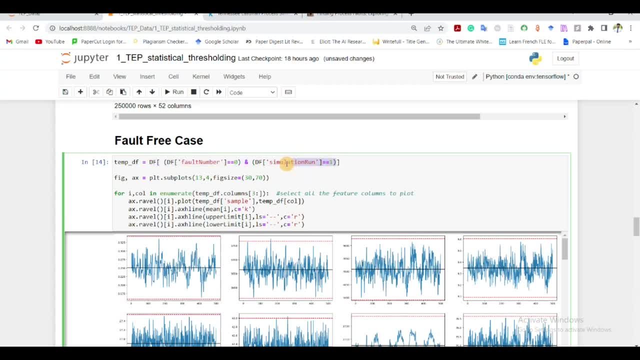 fault state. but right now i'm just importing the simulation run one. i'm not going to other simulation. will you can just change the simulation run value here, one to 500, and you can check for it, and then i'm plotting this. so first i'm creating a access which will correspond to 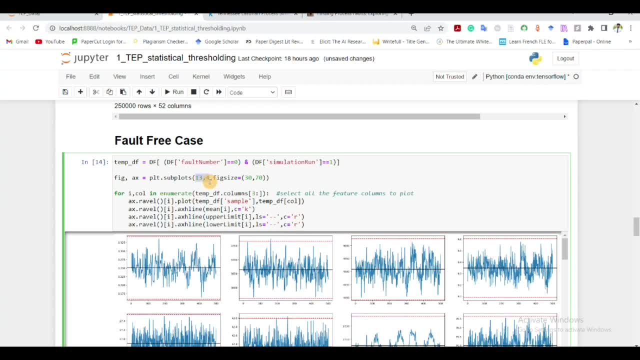 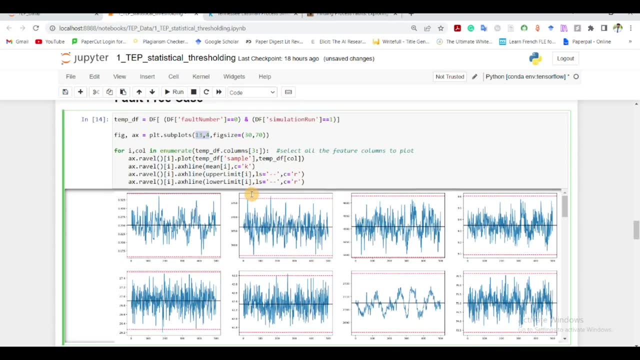 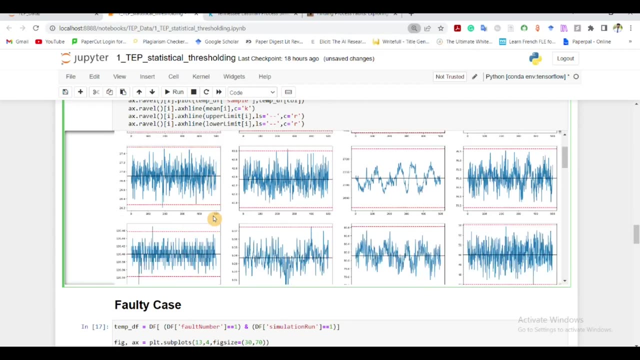 because i have 52 sensor value. i'm taking subplots 13 cross 4 and for each plot i'm going to populate with the corresponding variable. so what does so in this, all the variables? these are for one single run, single simulation run for 52 variables of the normal, normal health condition. 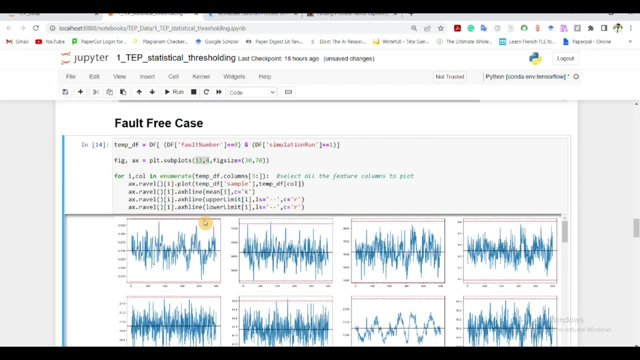 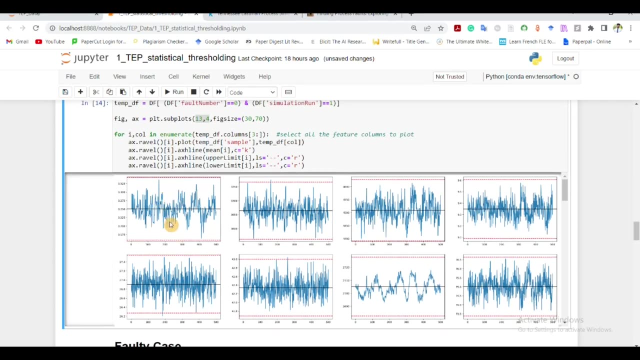 in normal fault-free condition. the red one belongs to the upper limit, the bottom red one belongs to the lower limit and the black one at the center represents the mean. so if the your process control, if the process variables, if this 52 process variables are within this red line, that means 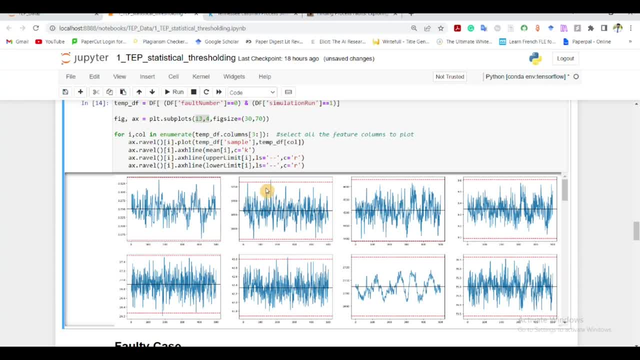 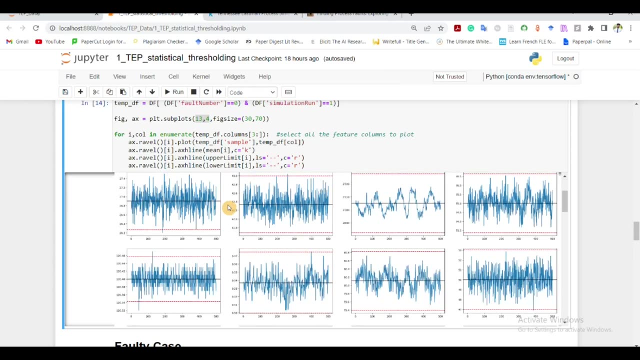 it's the normal condition. if they crosses this, cross this, like here you can see, though, it is a normal condition. there is some, uh, some uh, they're overpassing the threshold and giving us a false alarm, so that we need to consider also, and uh, here you can see. these are the 52 variables. 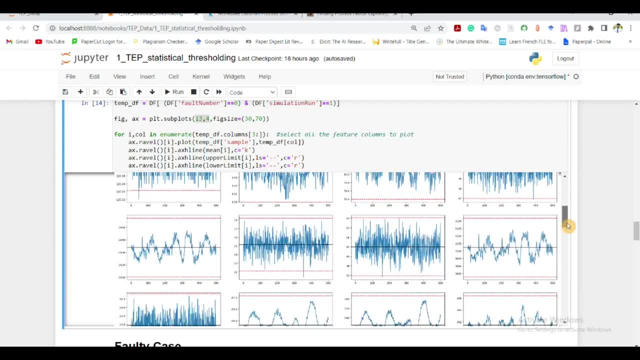 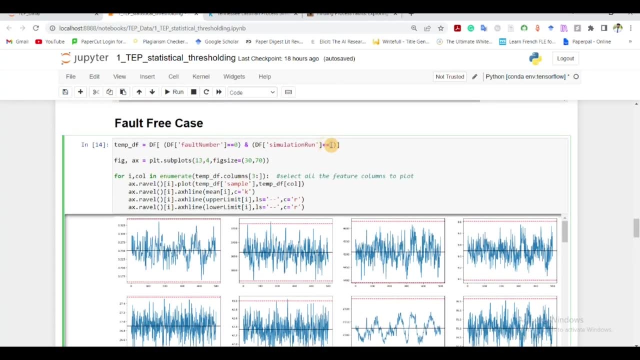 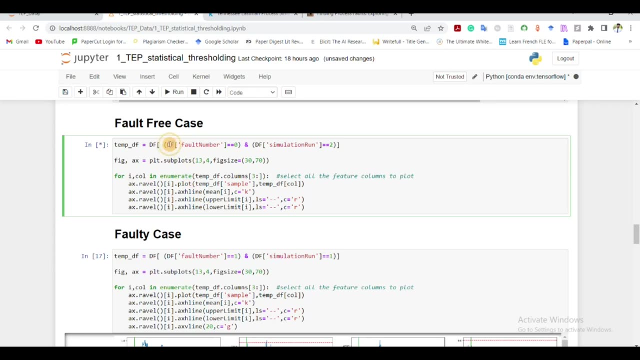 for one simulation run and most of them are lie within the within the defined upper limit and lower limit. we can do so. we can change that to simulation run 2 also. it should work fine. it takes a little time but no problem with that, because the df is a huge one. i think it's like 400 mb. yeah, for. 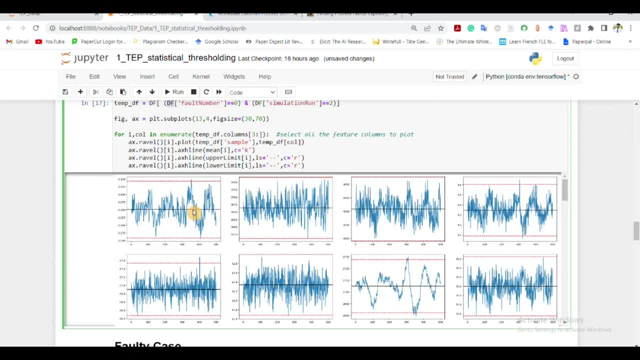 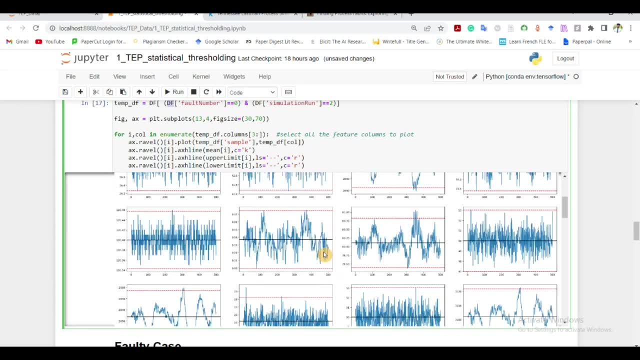 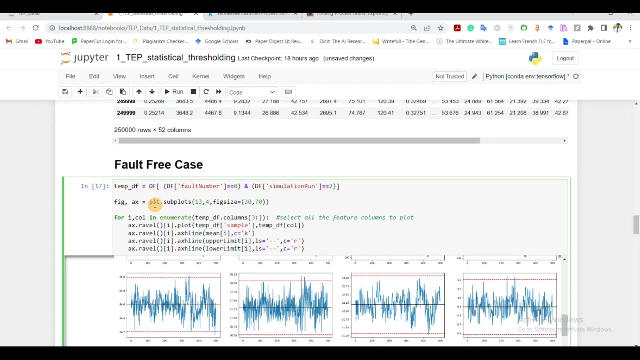 the simulation run 2 also, we can see that, yeah, most of like here it's under, here it's under the limit, here it's little outside the limit and things like that. yeah, you can check, but but the main idea is that they are mostly within the limit. so for now we can see that. 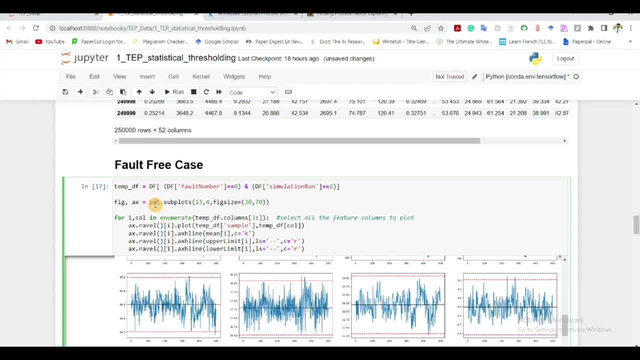 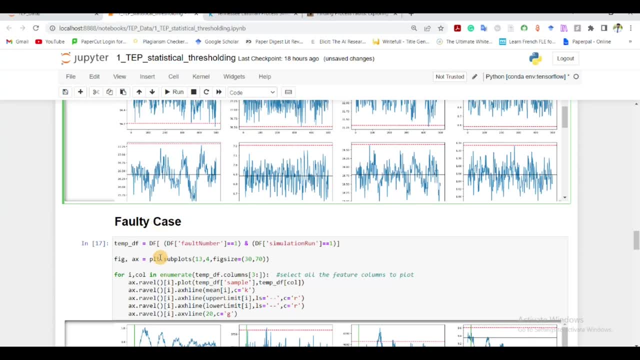 the statistical method that we have developed is well able to identify the normal fault condition just by using uh, normal distribution principles, and now it's time to see how it performs on a faulty case for the faulty case. what i'm going to do, i'm going to change, i'm going to 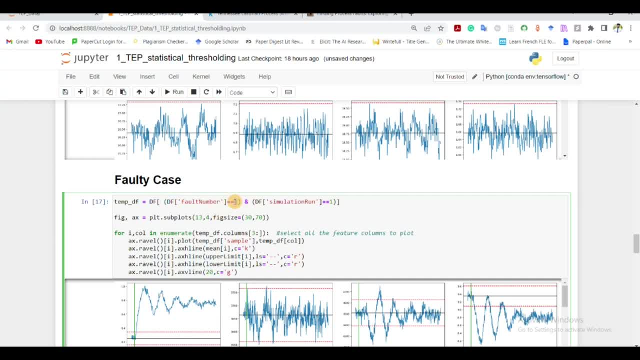 filter my data frame according to fault number one. that means the fault first false scenario or just one simulation, like the first simulation. it doesn't matter, you can change it and see, and i'm going to do same plotting, but right now what we can see is look at here the process. 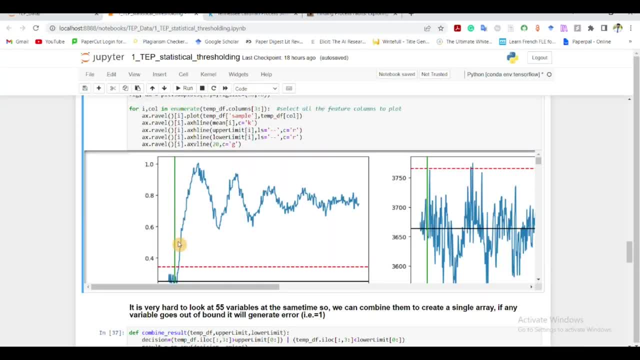 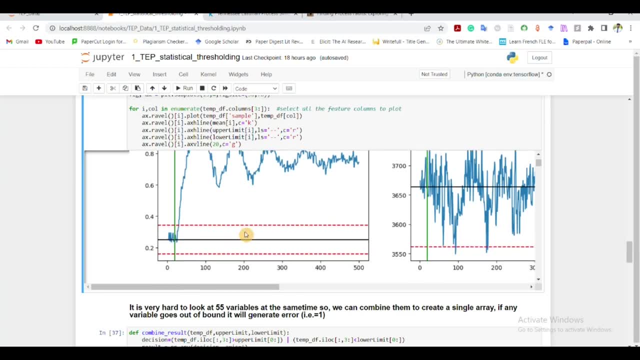 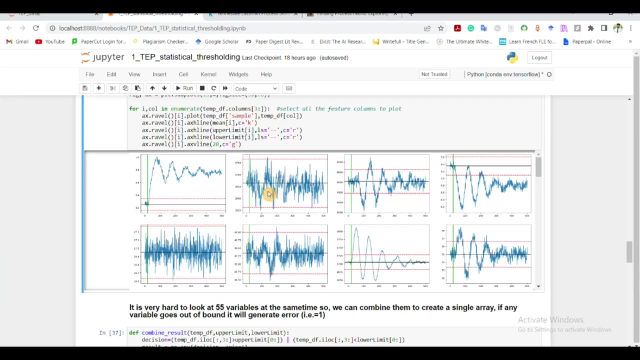 instantly deviates. uh, so here this green line represents the time when the fault was introduced, that is, the 20, and suddenly after that you see there is a deviation of fault that crosses the thresholds. so you can see: okay, there is a fault here, but but for the second. 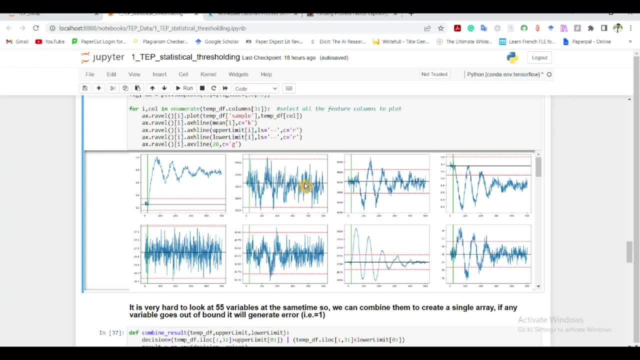 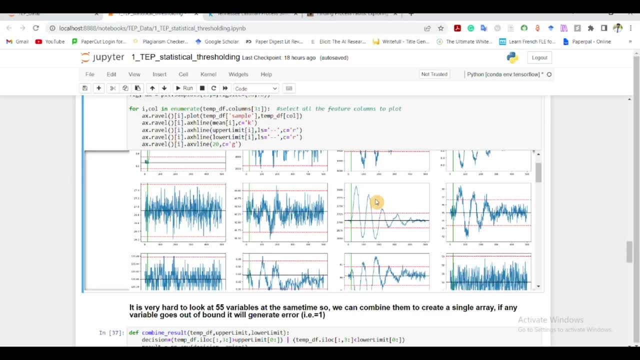 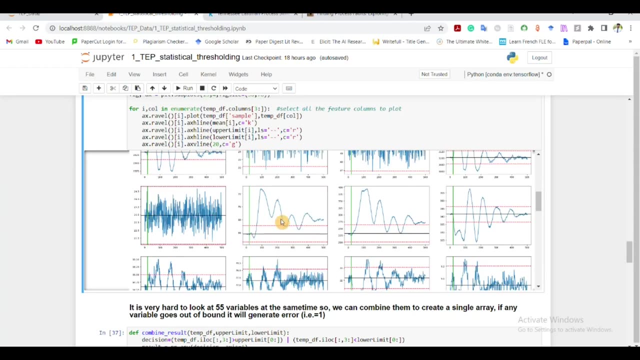 variable doesn't pass that much. so there are some variables which have higher impact on this kind of fault compared to other. so let's see, so this kind, this, this variable, you see it instantly surpassed the threshold, same as this one here, this one as well, this one as well. so, yeah, you can see. 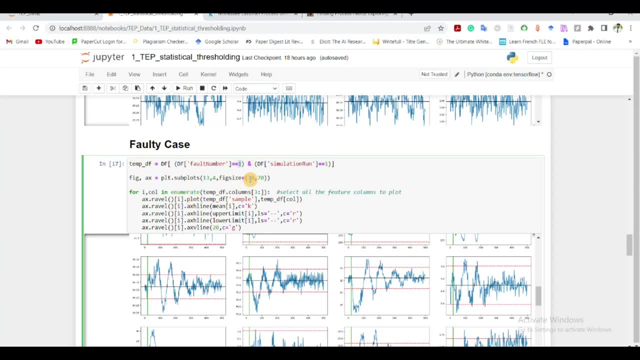 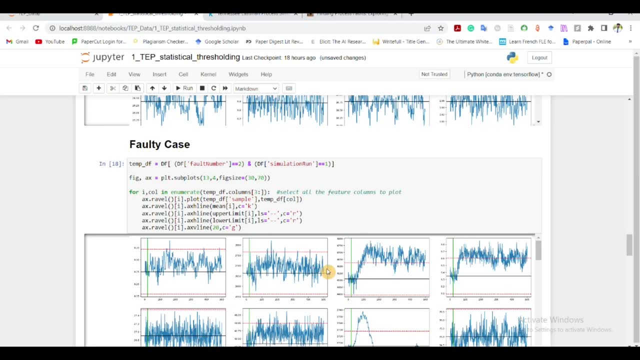 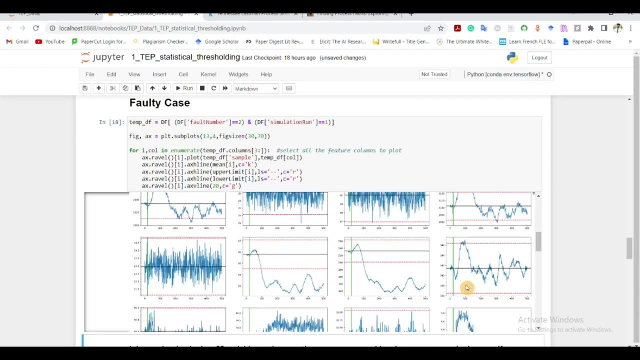 let's go and see, uh, some different fault. fault two: yeah, so also for fault two. yeah, here this variable surpasses the threshold and it can detect. we can detect fault two as well, just by using normal statistical method. but i think the fault three was the very difficult one. 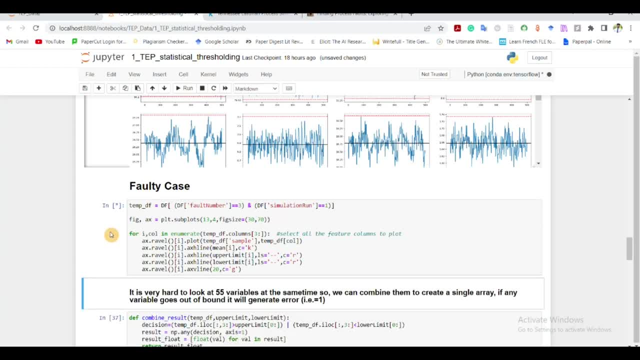 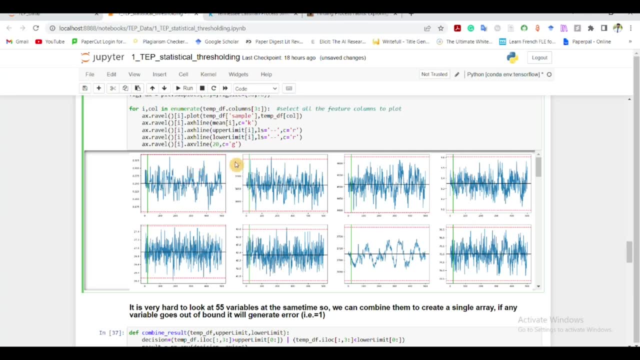 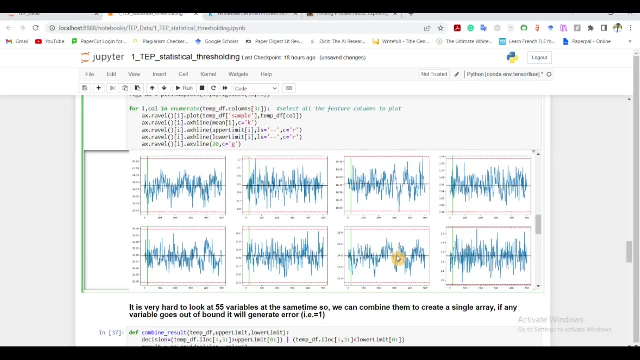 where it is. it's really challenging to detect that. compared to fault one for normal condition, the fault three is very similar. so let's see. so coming to yeah, in fault three you can see that most of the variables are lying underneath the thresholds. in fact, none of the variables are surpassing the threshold. 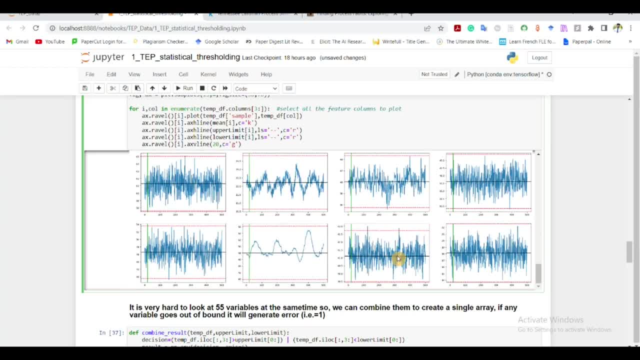 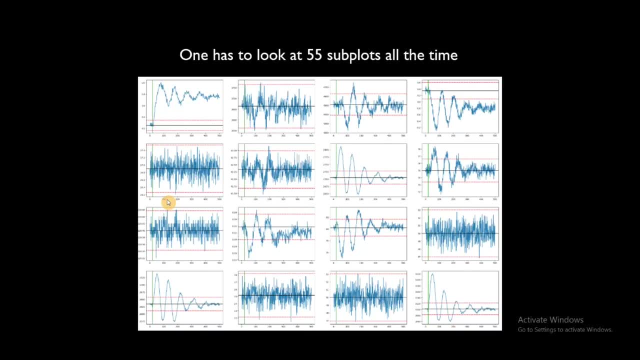 that we have already defined. so it's it's going to be pretty difficult to identify this fault just using statistical method, and also there is another problem that i'm going to discuss here is right now, what we saw is, for each case, we have to look at 50 to 55 or 52 different variables at 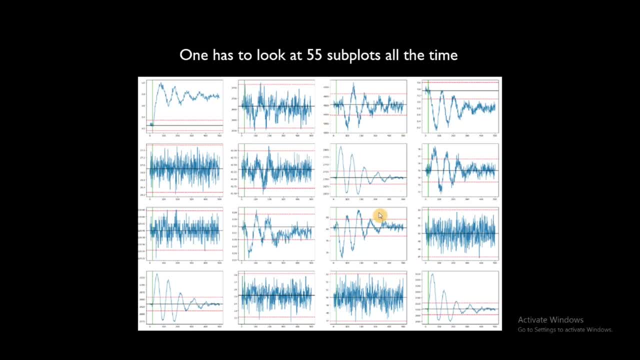 each time, which is not feasible for a human being to comprehend and look at all the 52 variables at one time. so what we want to do is, each time t, we want to combine this 52 variables, 52 variables, into single process parameter, so which will give us the 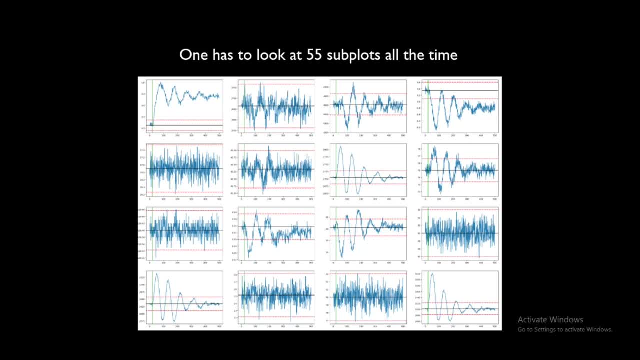 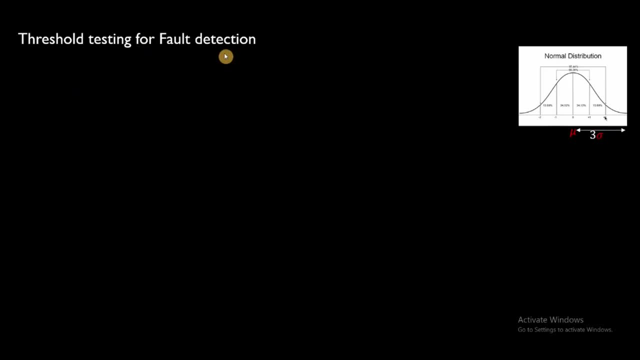 quality of the process going on at that time, whether there is a fault or not, and let's see how we are going to do that. so threshold testing for fault detection, this normal distribution curve, i put here, just for the reference, mu and three sigma. so what we have right now, we have the upper. 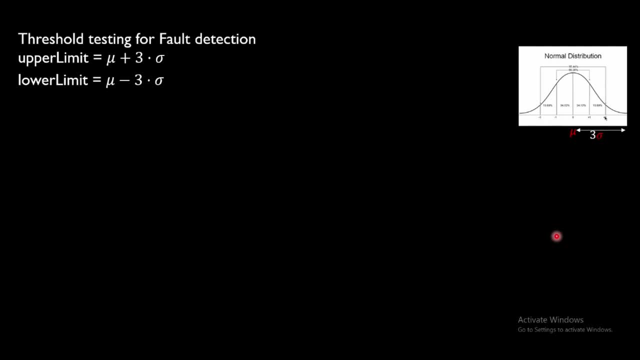 limit and lower limit value for all the different type of variables, sensor variables of the process. and let's say, we get a new variable at time t, which we need to do, which we need to say if this belongs to faulty state or healthy state. so at time t we get, let's say, 52 variable, 52 process variables, x1, x2 and x52. then what we do, 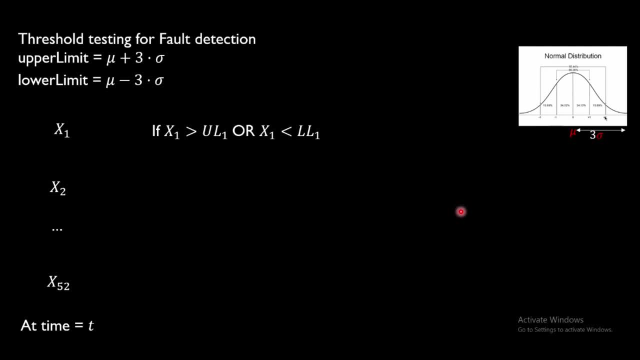 we do a threshold testing. what is our threshold? ul1 is our upper limit and ll1 is our lower limit. we need to check that if our this x1 variable passes the upper limit or it's lower than the lower limit, that will indicate, for if this is true, then it will indicate fault. 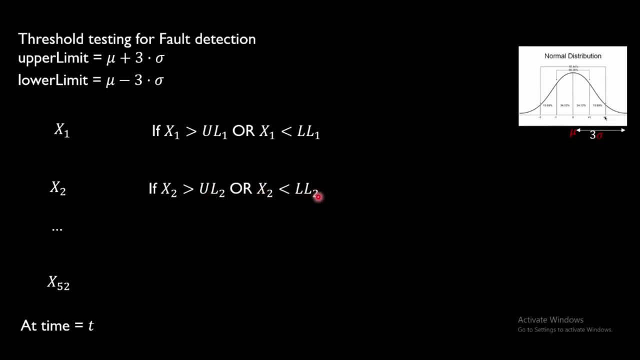 same we do for x2 variable. we have upper limit 2 and lower limit 2, and same for all the variables. so now what happened is this will give 1 or 0, 1 or 0, 1 or 0. now we can combine this all by using: 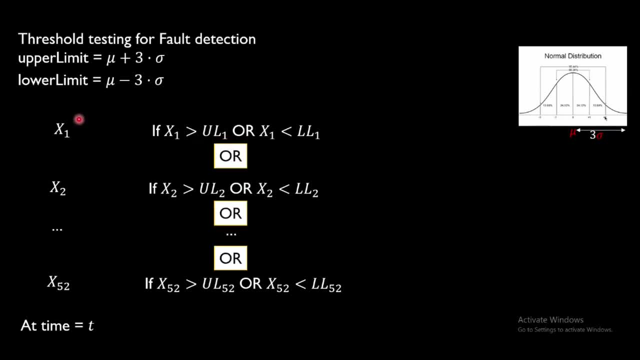 all condition, that means if any one of the variable has passed the threshold, indicate that there is a fault. so by using this simple method, we can do thiscomed. REPESEL method, difficulty swap method. so by using this simple method, we can combine these two. all Emirates are más and 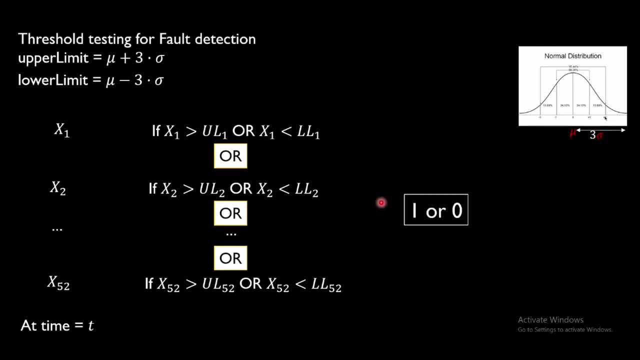 we can combine all the decision into a single method, So this entire part will output 1 or 0. Even if one variable has passed a threshold, it will give 1, because that's important for us, because the fault is important. 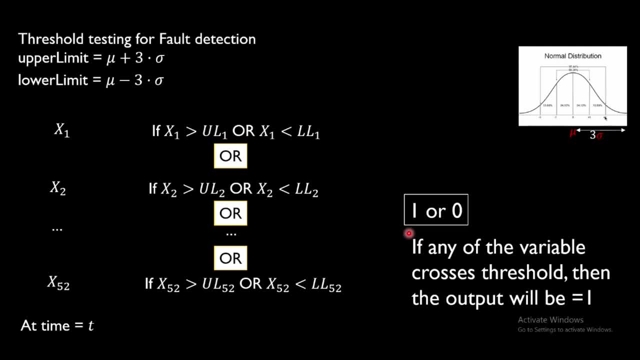 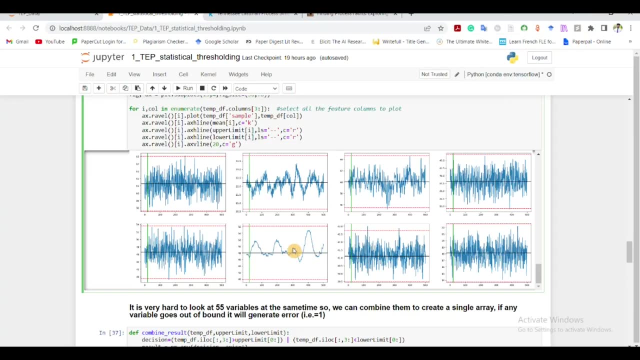 If there is a fault, it should not say there is no fault. So by using this simple method, we can combine the 52 variables decision into a single 1 or 0,, whether there is a fault or not. So now let's see how we can do that. 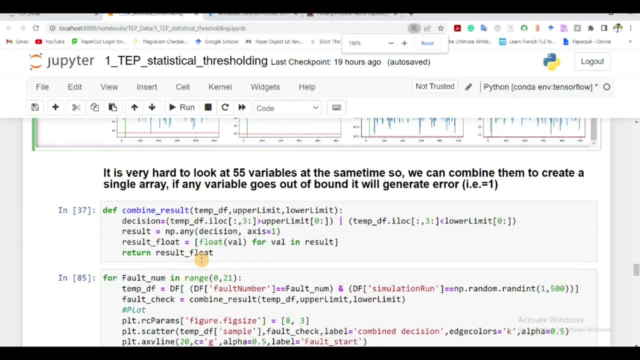 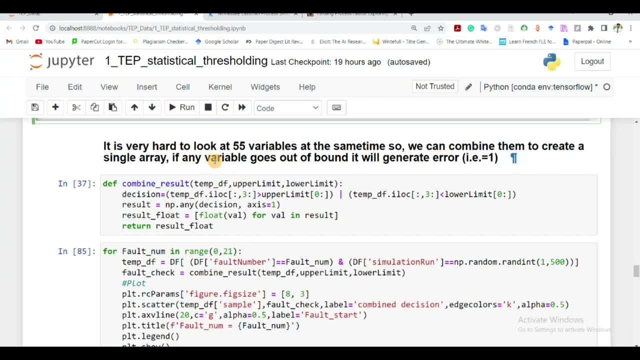 So for that what I did is very hard to look at 55 variables at the same time, So we can combine them to create a single array of any variable It goes out of one, it will generate one. That means there is a fault condition. 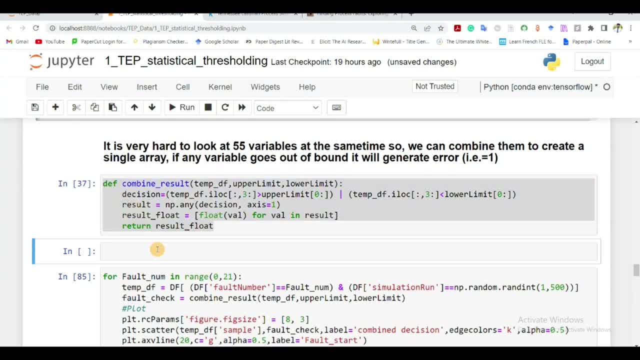 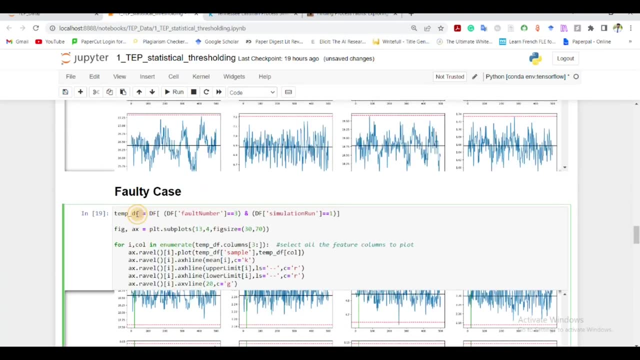 So for that I created this function. Let's see what this function does. So I have the temp tf. So this is the temp tf that I just created in this previous case, this temp tf from our different fault scenario. 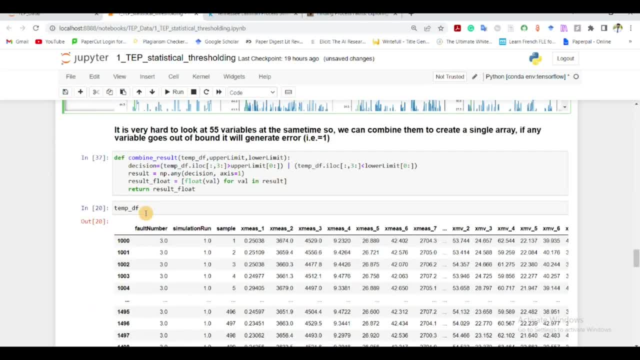 All right, So I'm using that temp tf and then what I'm putting my condition. The condition I show if it is greater than upper limit or it is less than lower limit, or condition in between, I get the decision And then using npany. 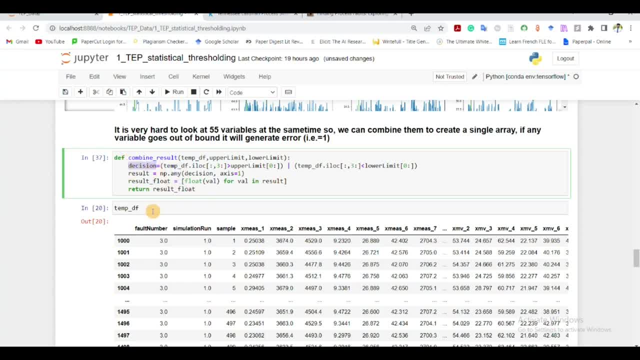 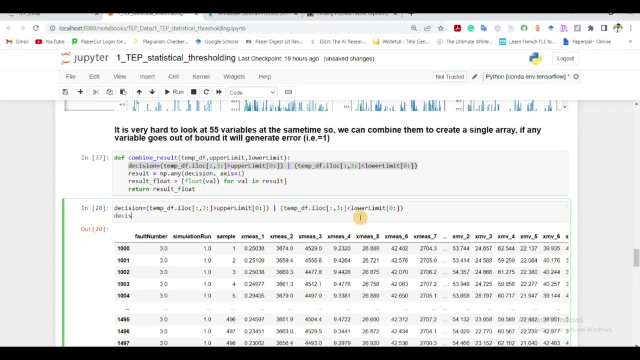 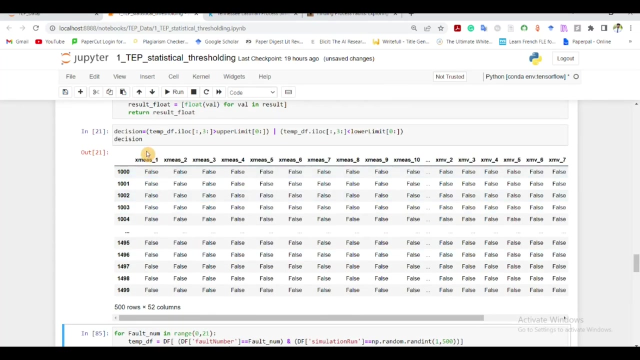 that will combine this decision all together. Okay, Let's see what does that mean, So I'll just copy and paste this one. So yeah, So now we did a checking like for all the variables, And then what we do. 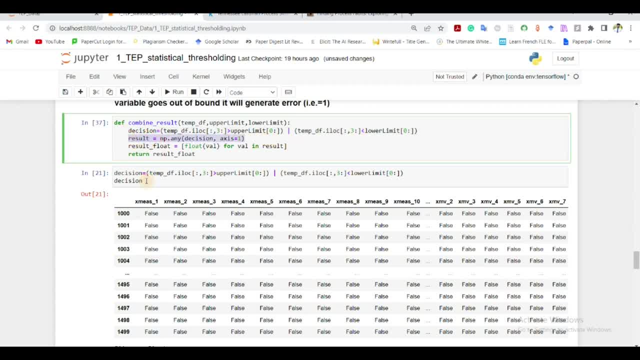 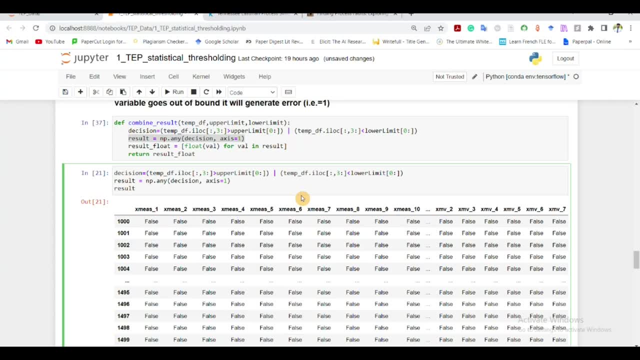 We do a check and paste here, So if the data is less than lower limit or condition in between, we get the result. So yeah, So now we see that for all entire 500, so entire length of the data. 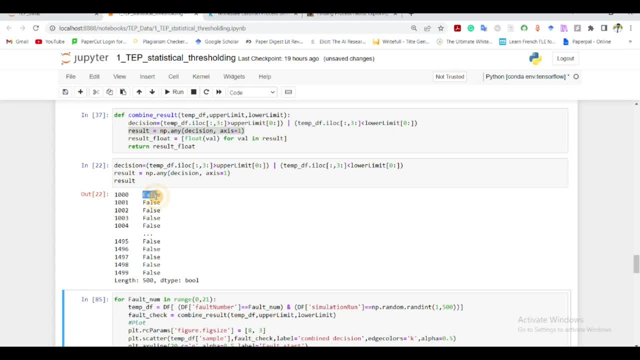 we get the final result: It says false. The statistical method says false for this condition. And then I'm just converting the Boolean value into full-of-flow. So that's fine. But if we convert it to a Boolean, we have another Boolean. 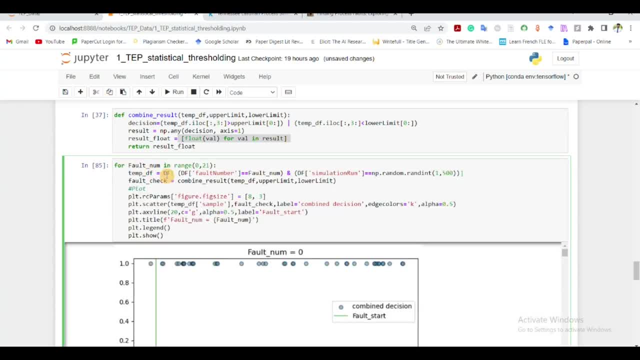 set. so i'm writing a for loop in this follow. what is happening is i'm going enumerating through different fault numbers. fault zero means the normal health condition and up to 20 like up to 20. this will exclude the last element and i'm going to in a temporary data frame, i'm going to 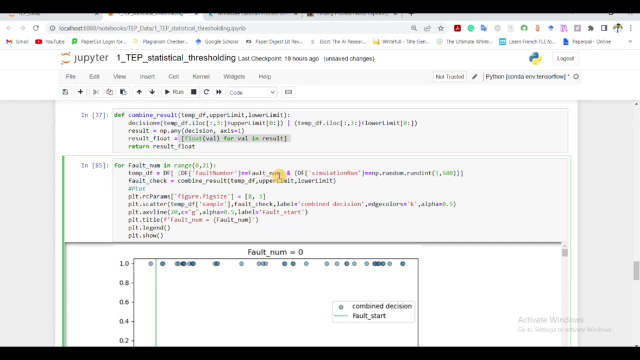 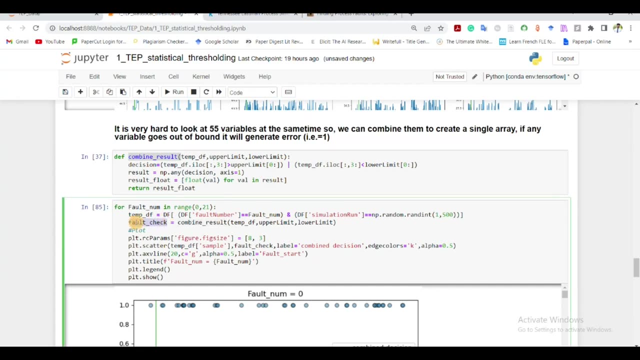 dump the value of that fault number and i'm going to see how the performance is. and this fault check is the result of this combined result function that we just created, so which will take the decision of 55 variables and combine it to one, all right. and then i'm just plotting it. and i'm just plotting a scatter plot. 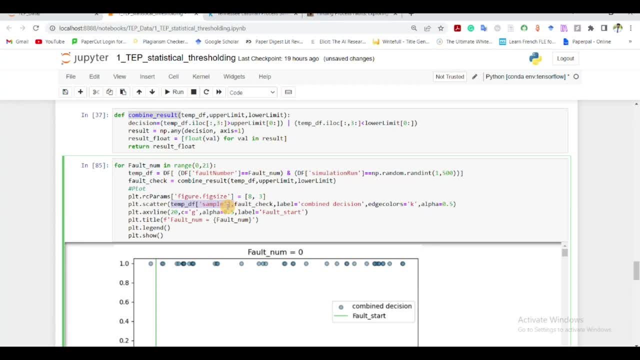 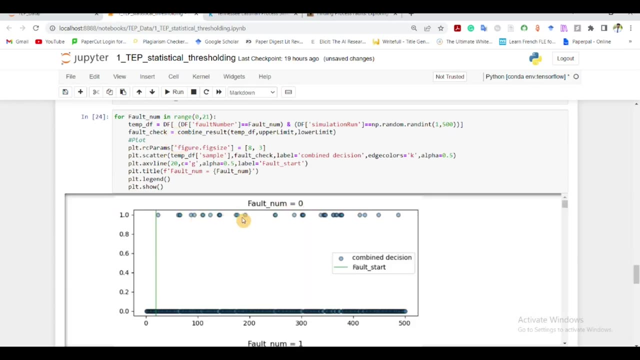 for the using the sample is x axis and fault check is your y axis. all right and all right, that's it. so now we can just run this one. so for fault number zero we don't have. we have some this false alarm rate that means there is no fault. but 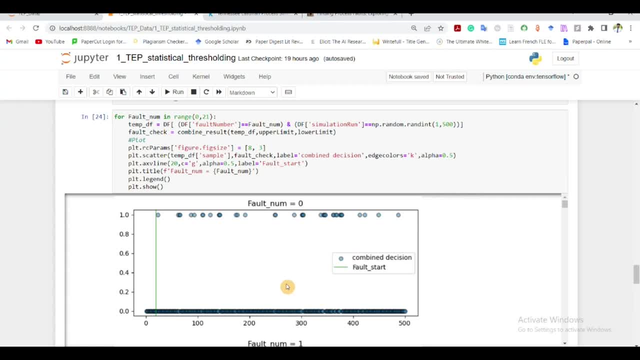 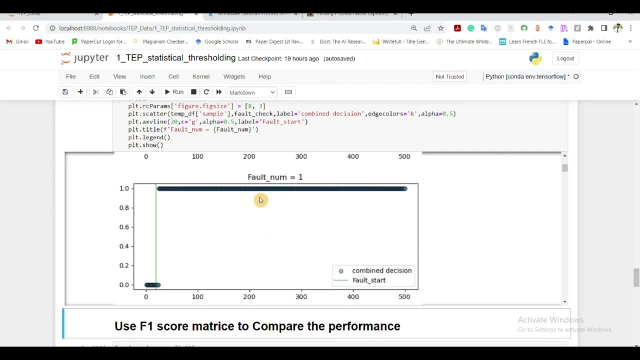 our algorithm is saying: okay, there is fault. so yeah, uh, this is one disadvantage of this method and uh, for fault number one, it's it's accurately able to identify. so, as soon as the fault has happened, the green line suggests when the fault has occurred- our algorithm is able to detect it. 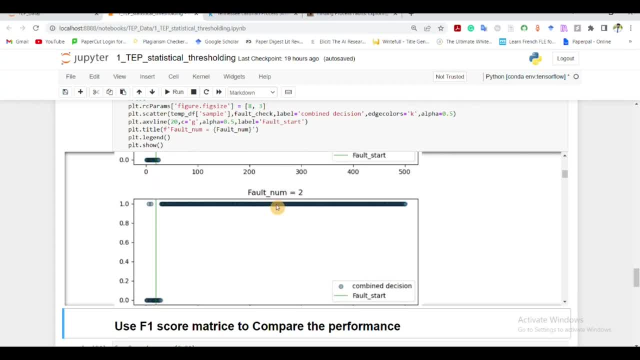 pretty accurately. for fault number two also, it's pretty able, pretty easily able to detect. but fault number three it's not at all able to detect. it's same, it thinks false three is uh normal fault condition itself. and for fault number four, yeah, very nice uh. fault five not that much. 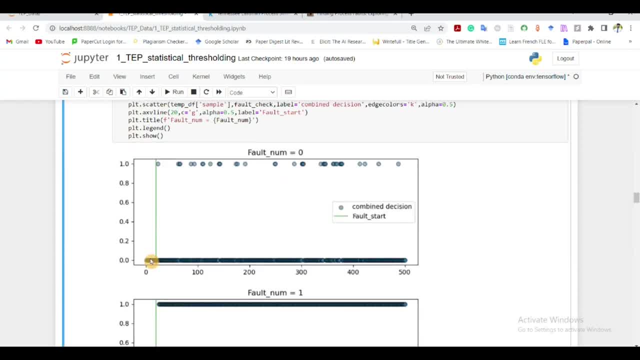 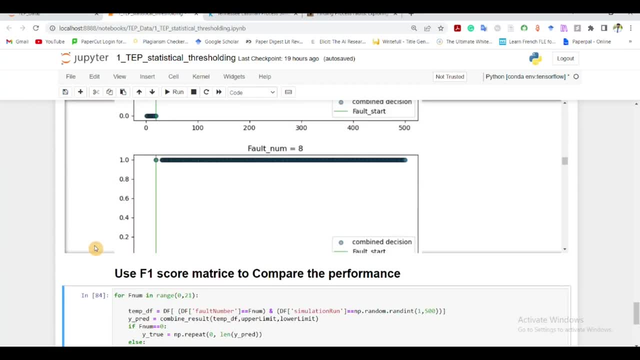 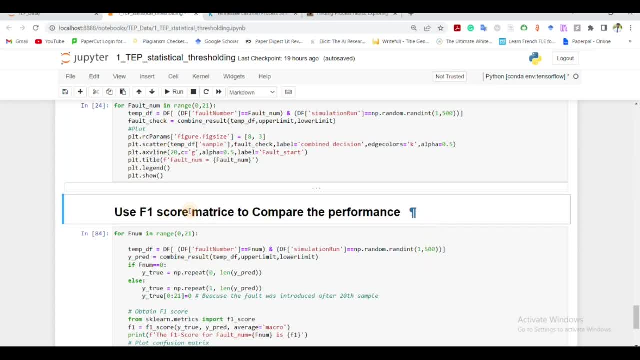 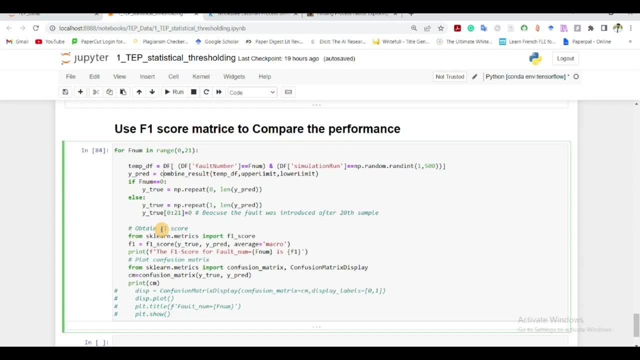 going to create a single matrix: f1 school. basically, this is a better accuracy matrix than comparing just the accuracy. that's what i want to say. all right, so what i'm going to do in this year is i'm going to write a function and i'm going to enumerate through uh for all the different type of 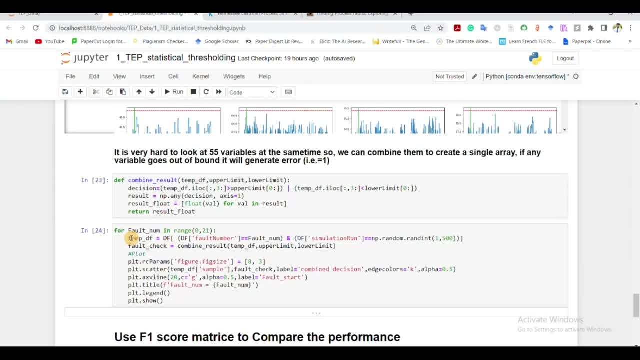 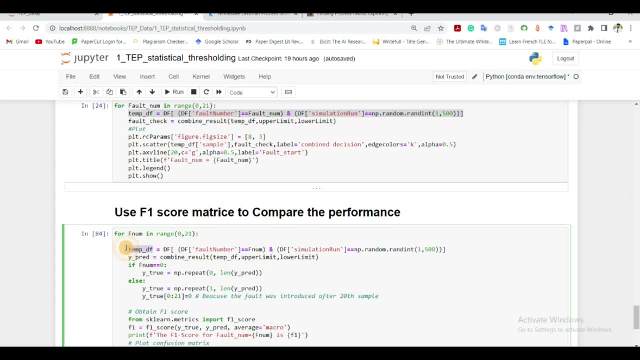 faults, the same one that i did here. the same one i did here is: i'm going to enumerate through different- uh, fault now- fault types. i'm going to put them in a file. yeah, for put them in a data frame. then i'm using the combined result to from the using the data frame, and it has two. 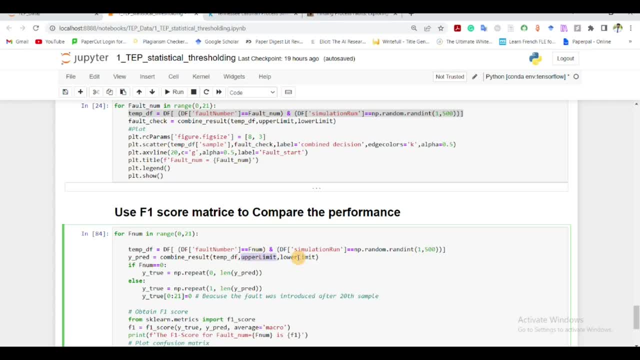 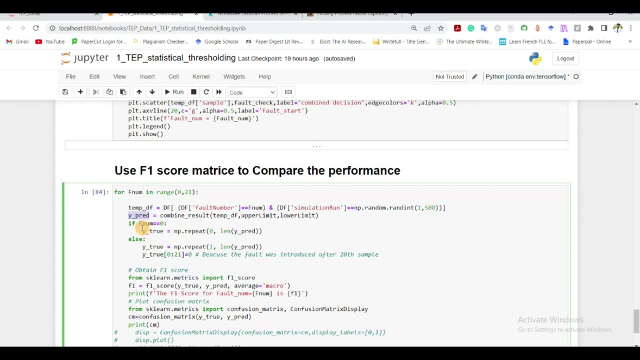 other inputs, so upper limit and lower limit to do the threshold checking and i get y pret, which is a single variable for each time instant. and i'm saying: if f num equal to zero, that means if it is the healthy condition, then my true, uh, my true label should be zero and else, if it 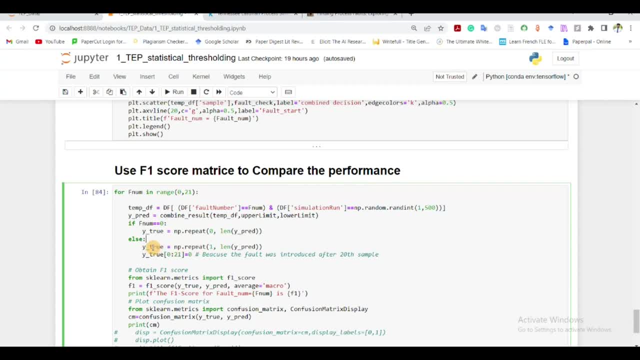 f num is not equal to zero, it belongs to any other fault, then my y true should be: uh, my y true should be one, but for the first 21 sample it belongs to zero because the fault was introduced after 20, after 20th sample, all right. so i thought this, this part is clear, and now let's see. now, now it's just. 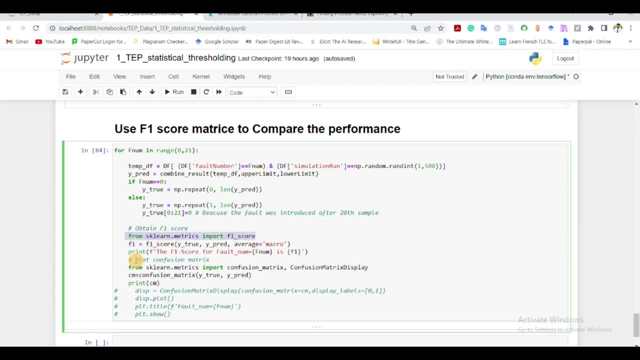 importing some uh matrices. so i import f1 score from a scalar, then i do: uh, true, this is the true, and this is the pred, the one predicted by my statistical method, and i'm averaging by macro and i'm printing the f1 score, then i'm just printing the confusion matrix as well. people who 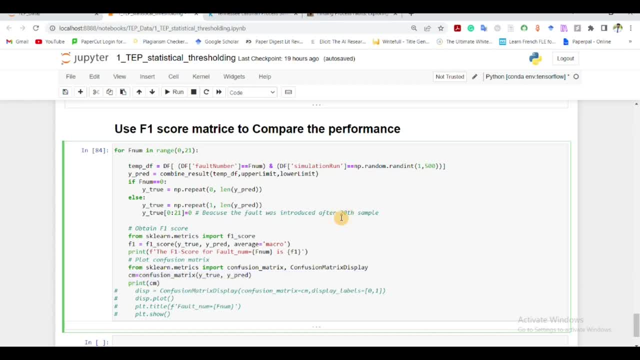 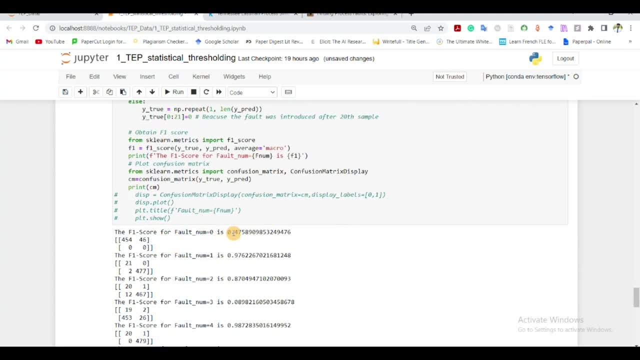 are acquainted with confusion matrix, it will be easier, so i'll just run this here. you can see that the f1 score for fault number 0 is 0.47. well, not that good, not that bad. the we can see that most of the zero condition it's able to classify, the fault-free condition has all the. 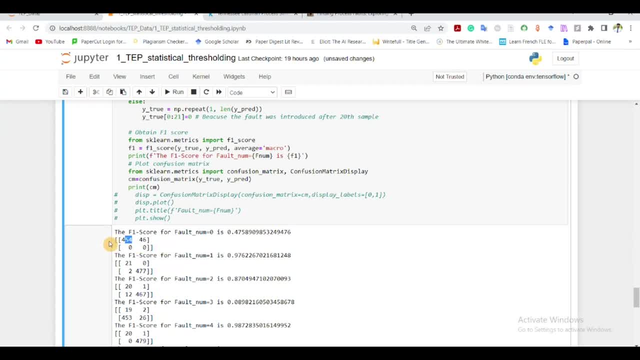 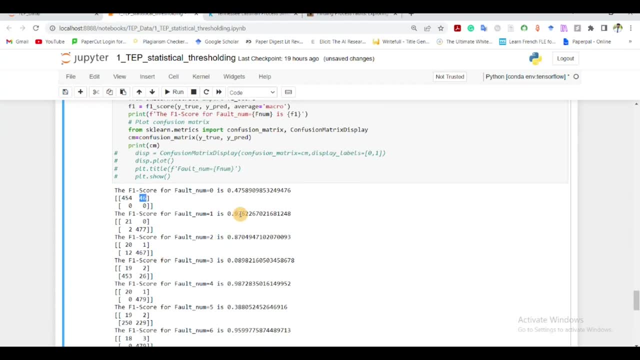 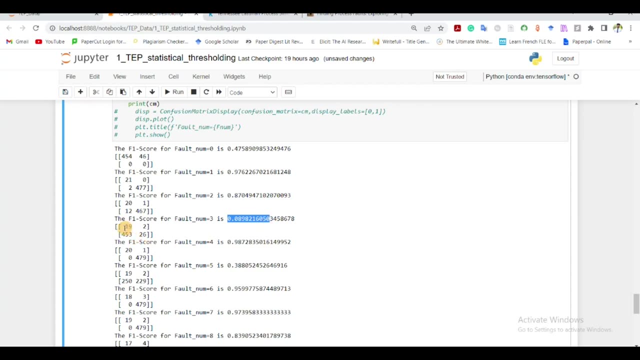 like there is no fault in a case actually there, so all belongs to zero. but there it is, predicting some cases as fault. okay, that we can, it's okay. but fault number one, we can see it has a very high f1 score. for fault two, it is very high f1 score, but fault three, it is very low performance. it's. 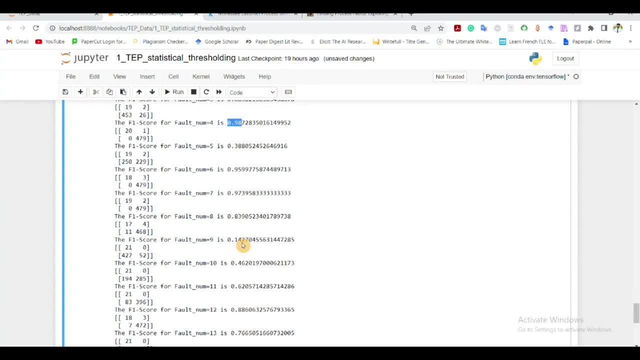 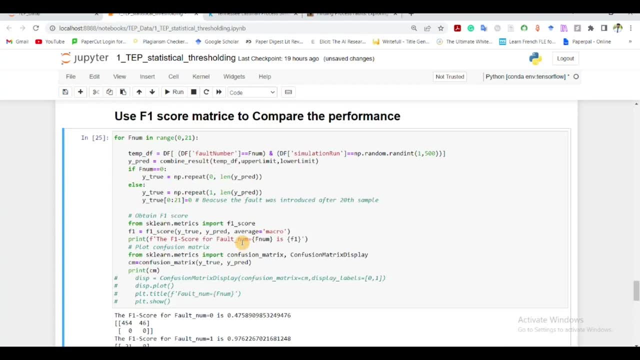 doing a lot of misclassification for fault four. yeah, very good, yeah, so basically we can see that there is there is pretty good performance just by just by considering the statistical method. that was all about this video, and in the next video we are going to use principal component. 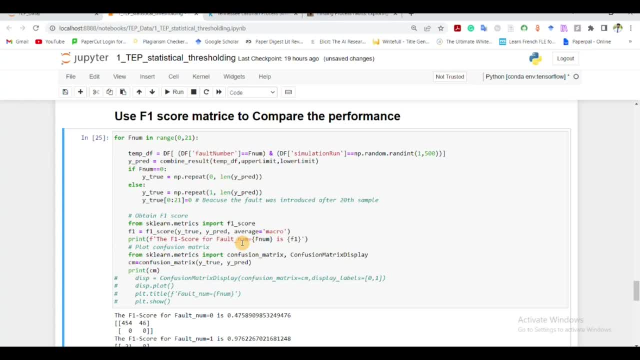 analysis in an unsupervised way to do anomaly detection. so yeah, i hope i'll see you in the next video.